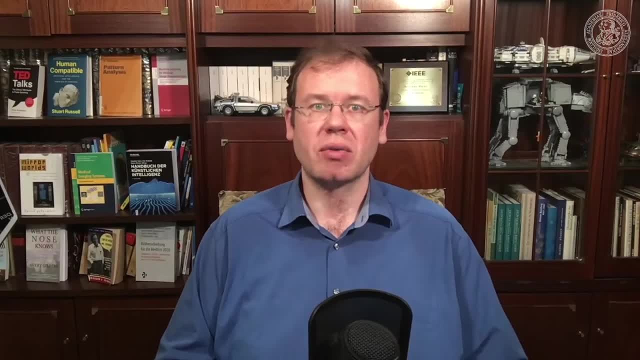 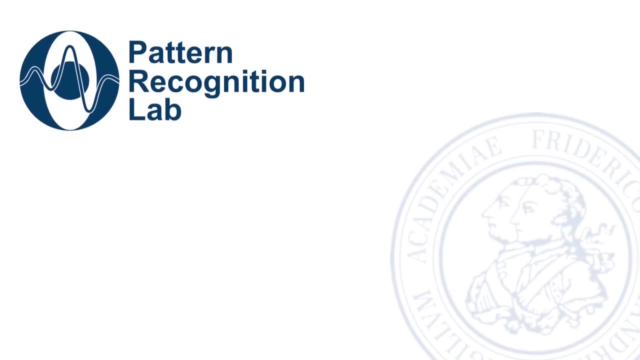 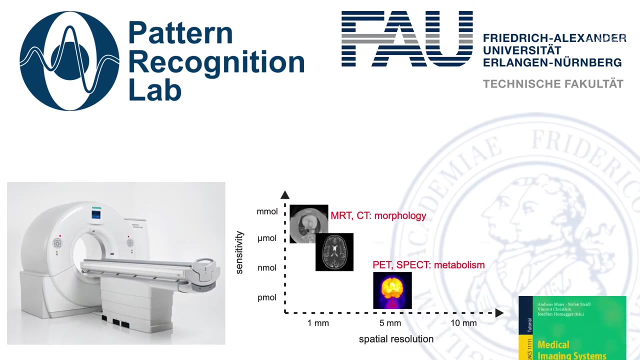 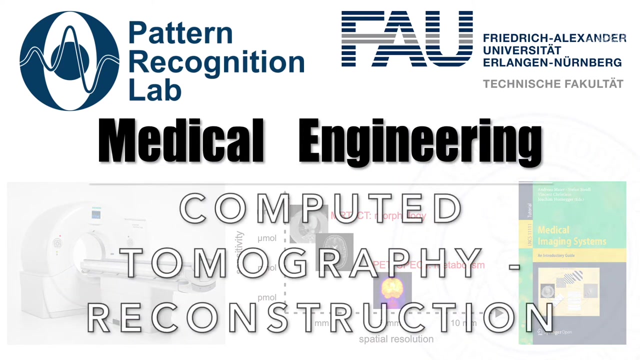 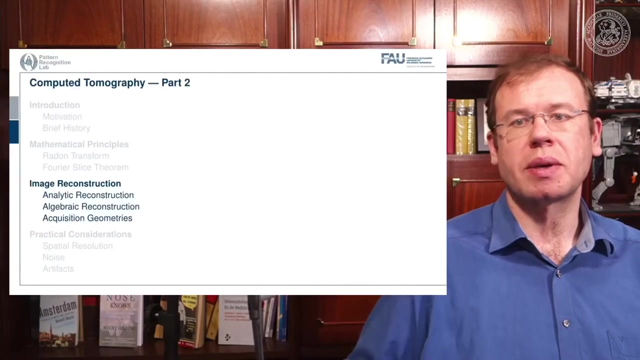 looking forward to be looking into the reconstruction algorithms of computed tomography. So here we see how we want to proceed with the reconstruction algorithms, And today's topic is the reconstruction algorithms of computed tomography. So these are essentially the main reconstruction families. There is the analytic reconstruction. 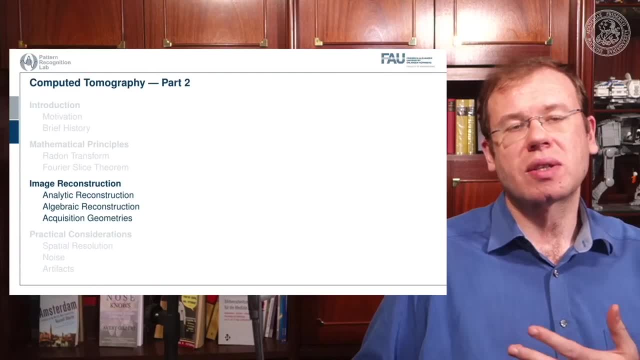 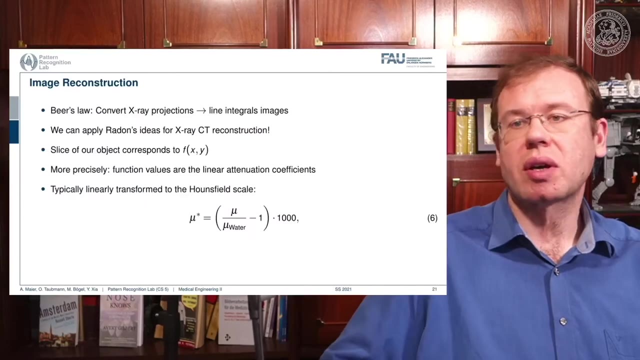 and the algebraic reconstruction, And there's also a couple of changes in acquisition geometry that allow us to make much faster acquisitions. So these are the main topics that we want to discuss in the video today. Now let's go ahead and have a look at the reconstruction problem. 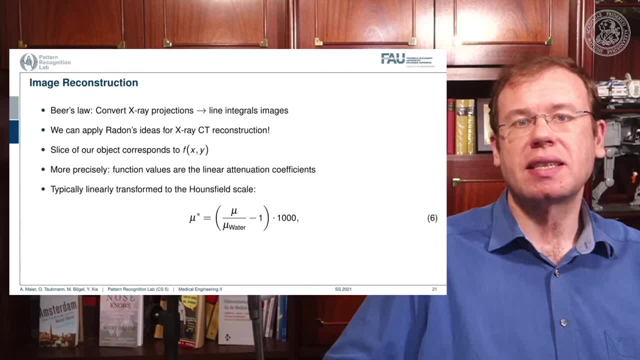 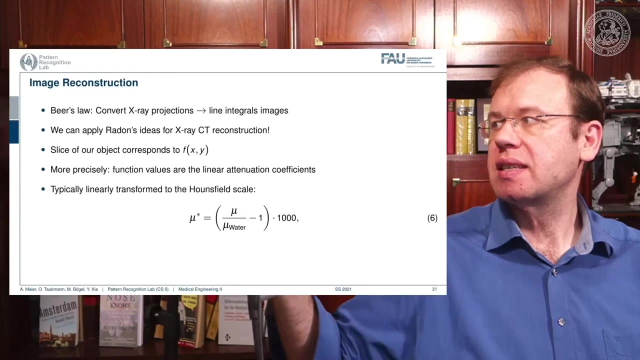 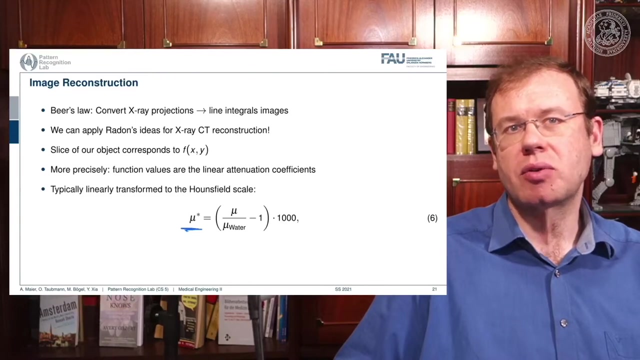 One key problem that we have is that the x-ray projections- they essentially form line integrals And we understood how we can essentially get the original information, But what we still haven't discussed is that this mu- they're actually dependent on the x-ray energy, So we somehow want to be able to create standardized values. 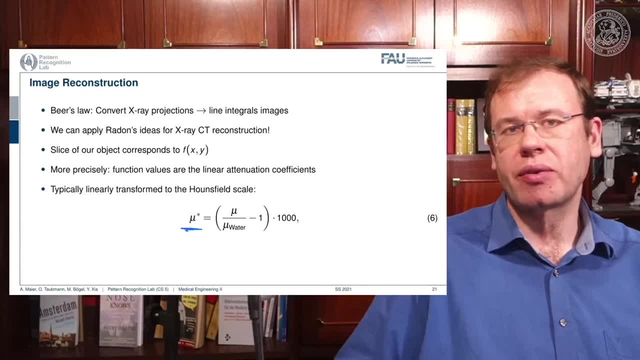 And this is why in reconstruction theory we have introduced so-called Hounsfield values. And the Hounsfield values now standardize the absorption coefficient that we know is energy dependent And they divide it by the absorption coefficient of water minus one. So if you have water, this would be exactly one. 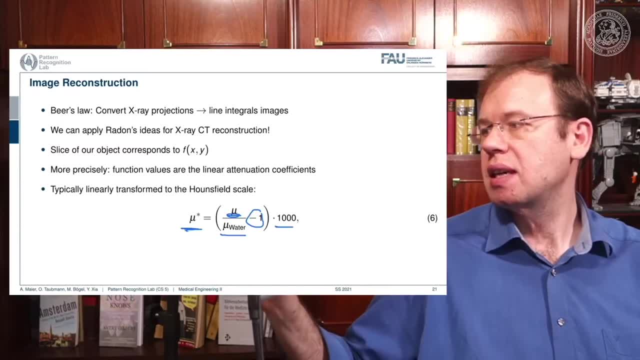 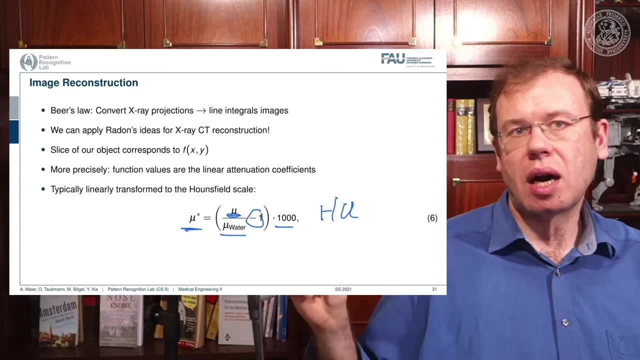 you subtract one and then you multiply with 1000. And the unit is then given as Hounsfield units. H? u Now the Hounsfield units, they have the property that they're exactly zero for water And they're minus 1000 for air. So these are essentially the two points: air or no density. 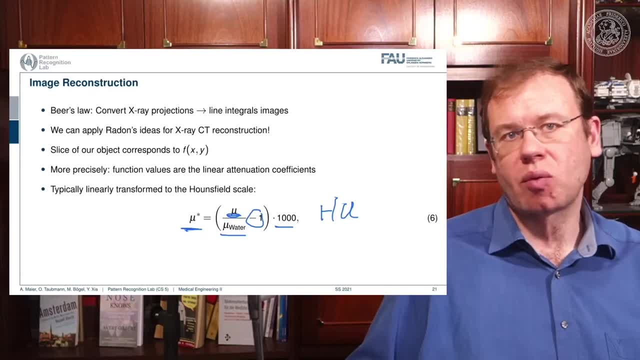 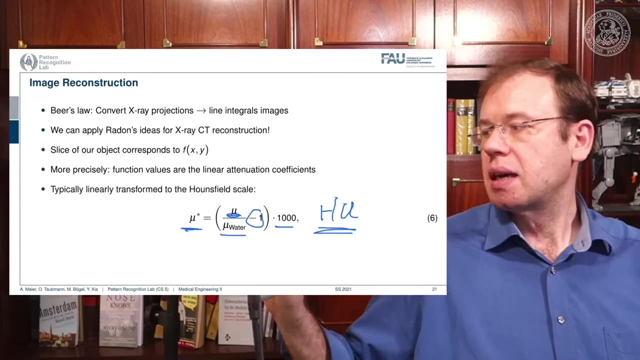 would be zero And water would be exactly one after the scaling, And this means that we have a kind of standardization for water And, of course, water is the most important material inside of the human body. This is why this kind of scaling has been chosen. This comes at a couple of interesting 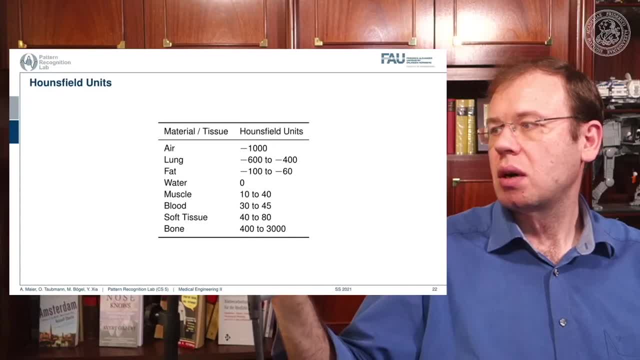 effects. So, first of all, the standardization only holds for air with minus 1000. And for water with zero. For all the other tissues, you see that we have different kinds of value ranges: for the lung, minus 600 to minus 400,. 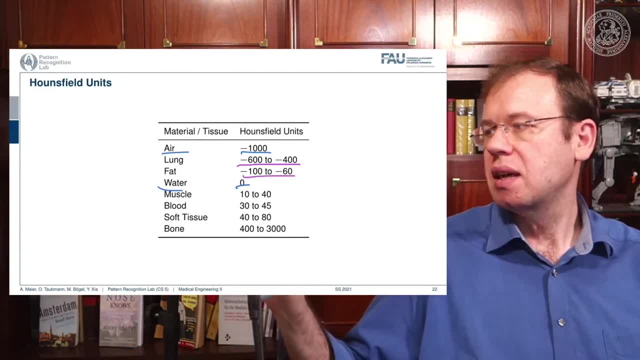 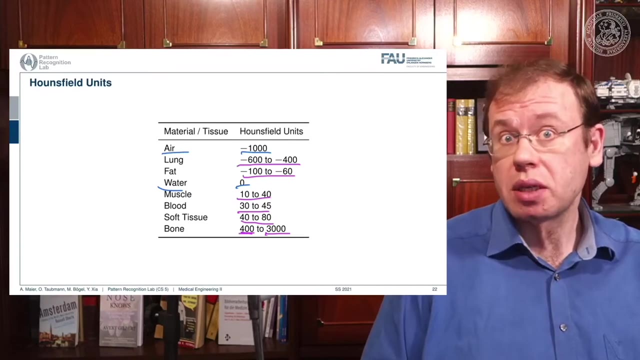 for fat to minus 100, to minus 60.. For muscle, then we have Hounsfield values that are higher than zero, And bone, we are in the range between 400 and 3000.. Now, why do we have actually these ranges? First of all, the human tissues, and the human tissues are, of course, 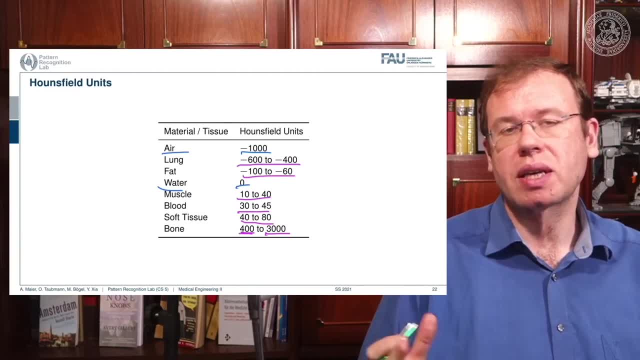 variable. So not every human is built in the same way And we can easily standardize for water and air, But for human tissues it's more difficult. And second, depending on the choice of your acceleration voltage and the x ray acquisition, you will have a different nonlinear effect on. 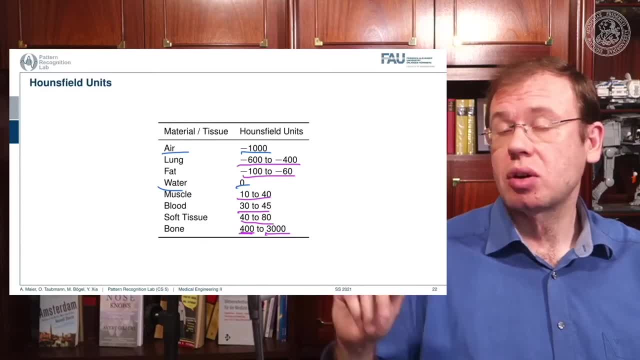 the actual Hounsfield units. So the standardization only holds for water and air and all the other Hounsfield units that are generated from this they are dependent on the actual acceleration voltage of the imaging process, So you get a different contrast. 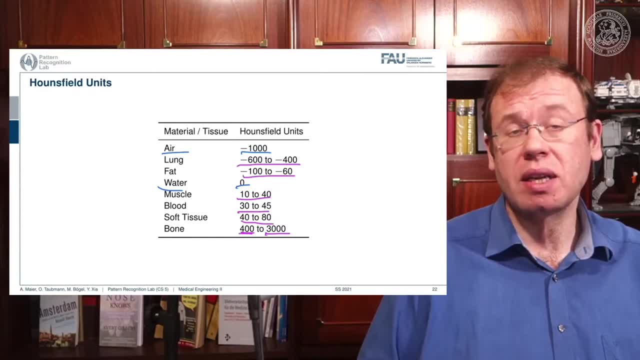 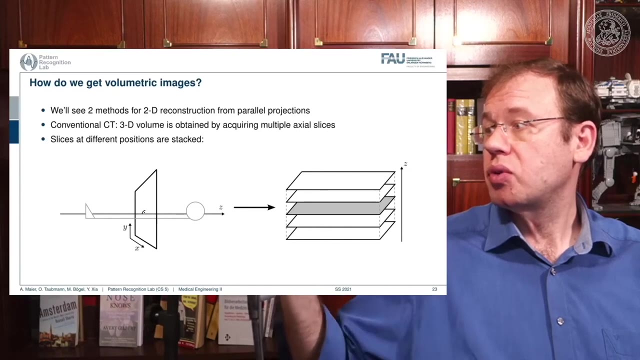 if your image at 120 kV or at 80 kV, the images will appear differently, And this is also what than gives rise to this. ranges of Hounsfield units. Now the next thing is: how can we get volumetric? 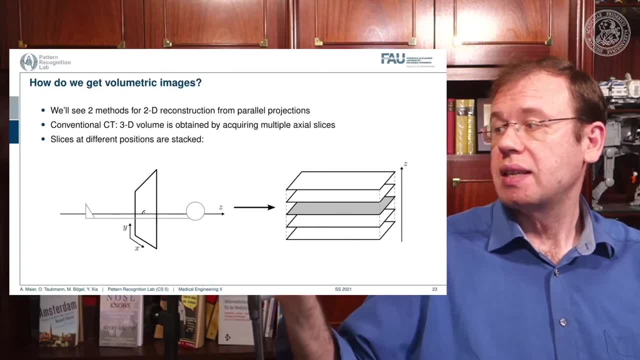 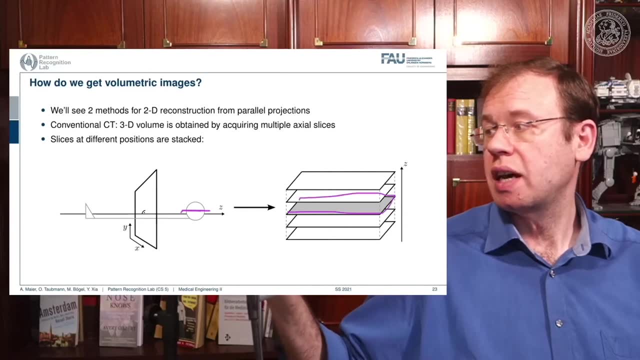 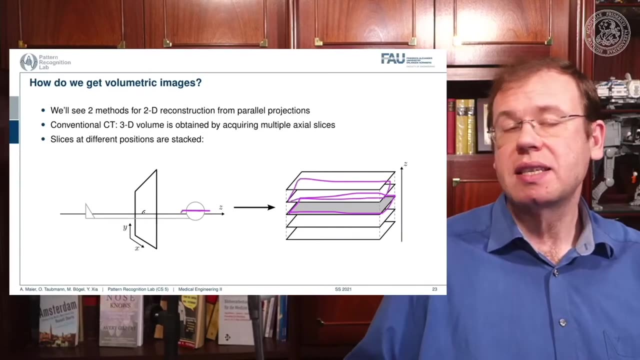 images. And yeah, you see, here we had a kind of object. we don't want just a single slice, but we only understand how to reconstruct one slice here, but obviously you can stack this. yeah, so i can just repeat the acquisition and this is how actually the first scanner by hansfield and kormak was actually. 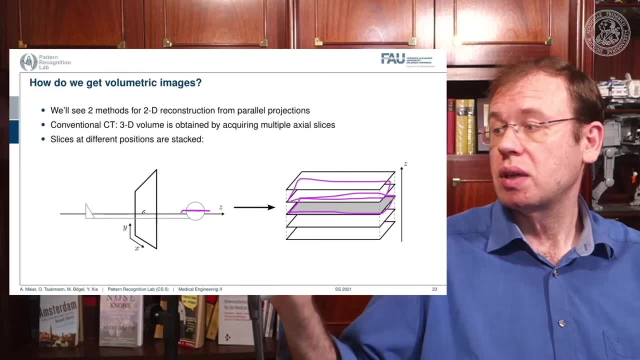 working. it really had a line element, so it was only acquiring a single line here, and it had a detector. that was even more difficult because it actually had just a single source element and then also a single detector element, and what they did is they translated them in order to build an entire. 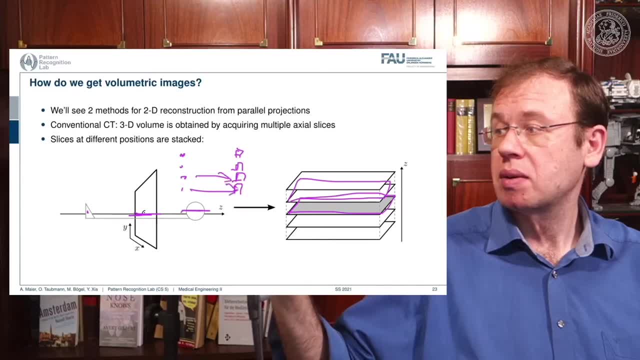 acquisition. so this was really a parallel beam acquisition like this one here, and they needed to shift here in order to construct the image and then if you want to construct the next slice, you have to shift essentially you into the set direction. so you now essentially shift. this is the 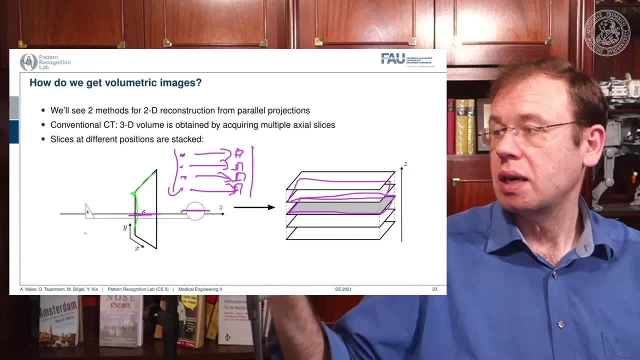 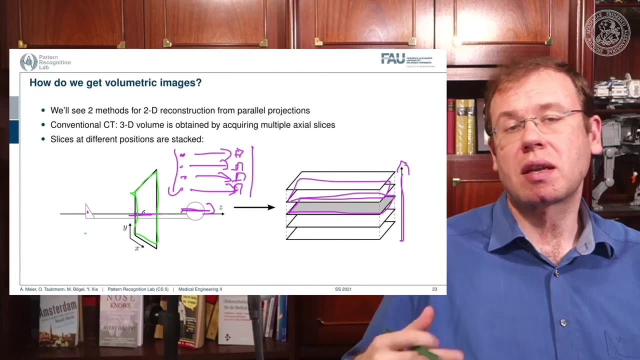 acquisition plane. so this is xy that we've seen previously, and now i take it and shift the entire thing into the set direction in order to get multiple of those slices. so that's the key idea: how we can get to volumetric images. and now you also. 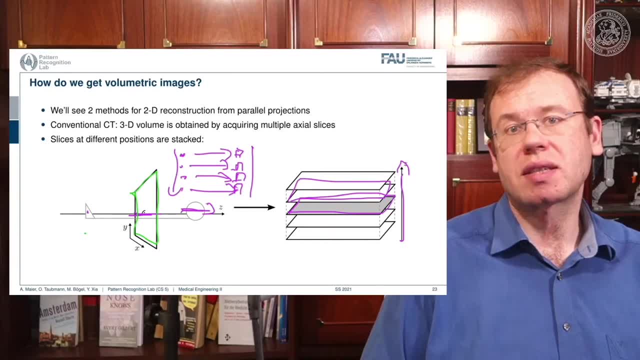 might understand why it's a cool technology to have a helical scan, because then we can do the acquisition in a continuous mode. here we have to stop acquire, shift, acquire and so on, so this takes a long time. so this is also the reason why the original scans took so long. with the modern systems we can be much. 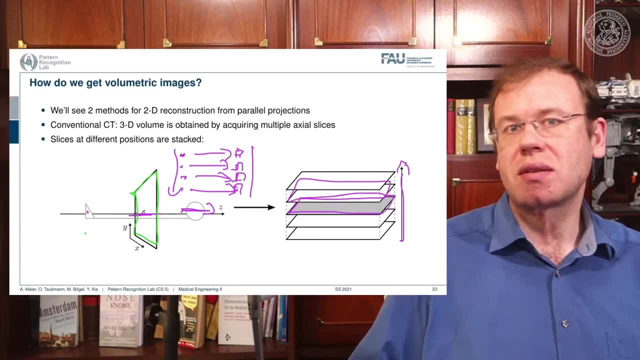 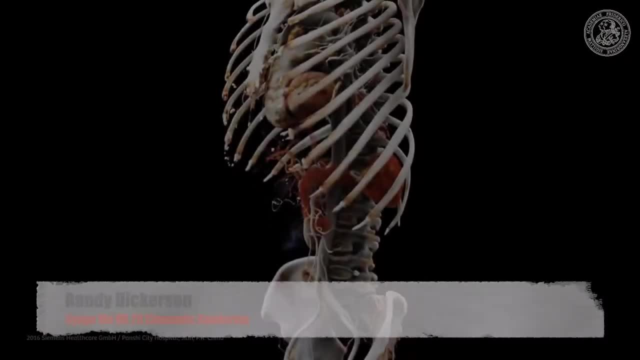 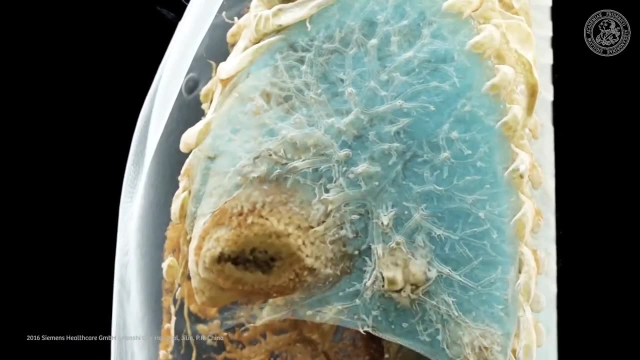 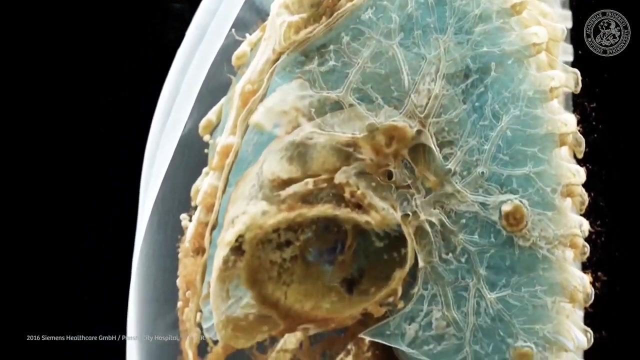 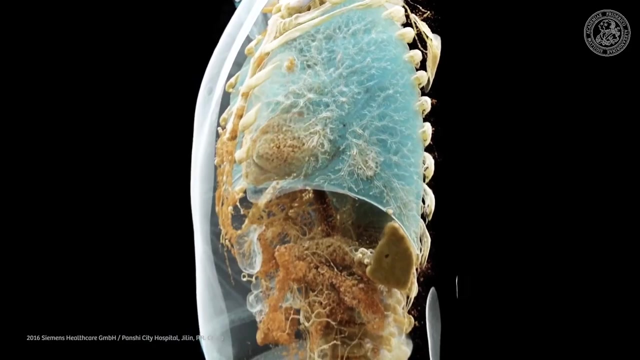 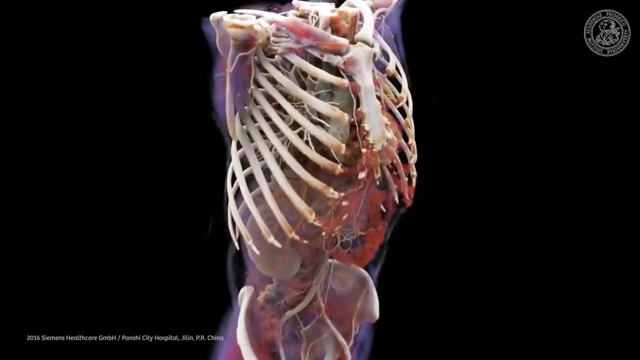 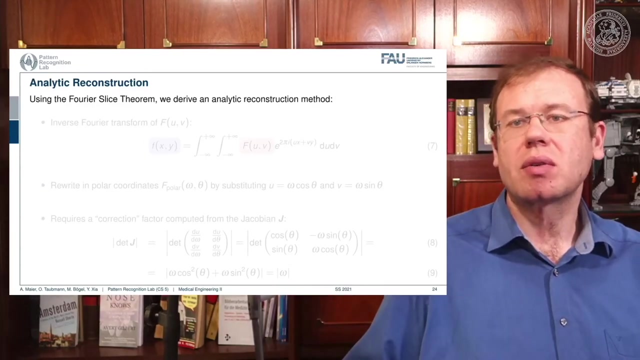 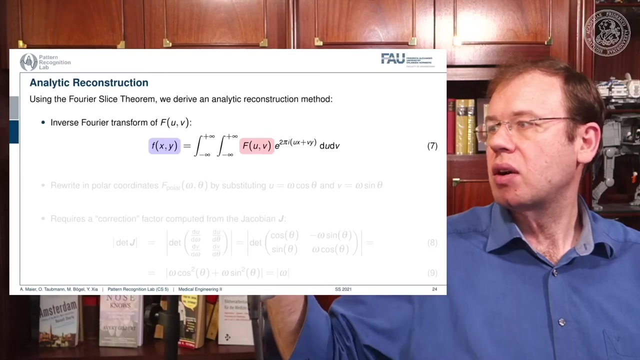 faster because we discovered the continuous effects of the different motions involved. here also, we are using very different detector technology. so now, how would we then derive a reconstruction algorithm? and we can use now the fourier slice theorem to derive an analytic reconstruction method. so the key idea is that we start with the inverse fourier transform of our 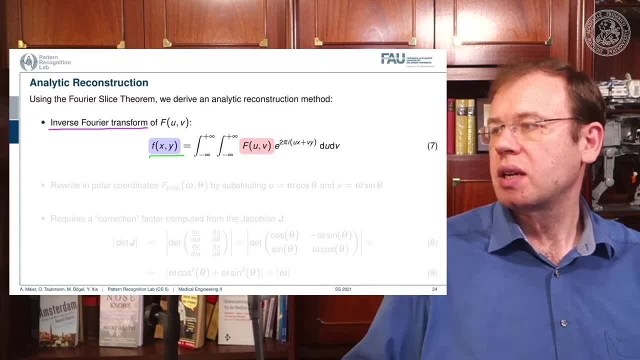 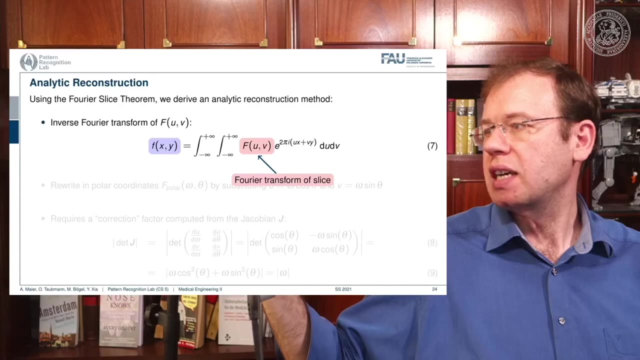 object. we've already seen that the object can be given as f of x, and if we had the entire fourier space, then the inverse fourier transform would solve the entire issue. now if we want to do that, then we need the fourier transform of the slice and we will get the reconstructed. 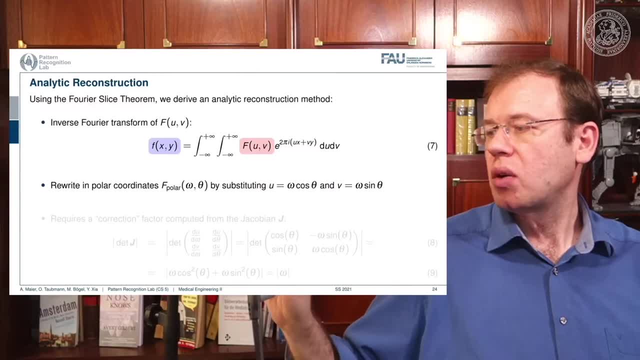 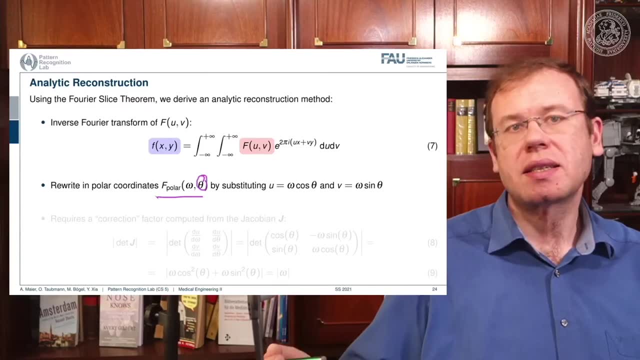 result of the fourier transform of the slice. so what we do in order to get an efficient solution is we use polar coordinates where we have the angle feeder in here, and this is very important because we're actually acquiring on a polar coordinate system. right, because we are rotating the 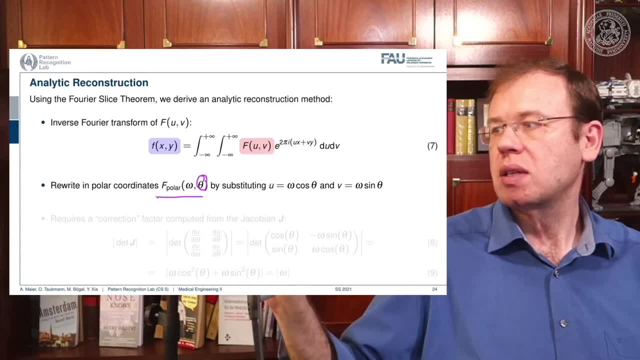 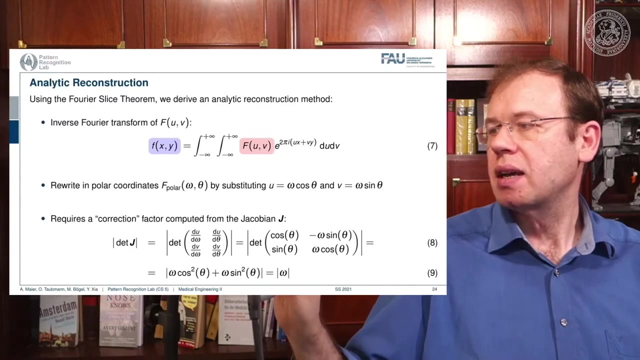 detector about the patient, and we are dependent on this angle feeder here, and this can be done by substituting you with these polar representations here, and, if you want to do so, this is also something that you learn in mathematics- that requires a correction with a factor that is computed from the so-called 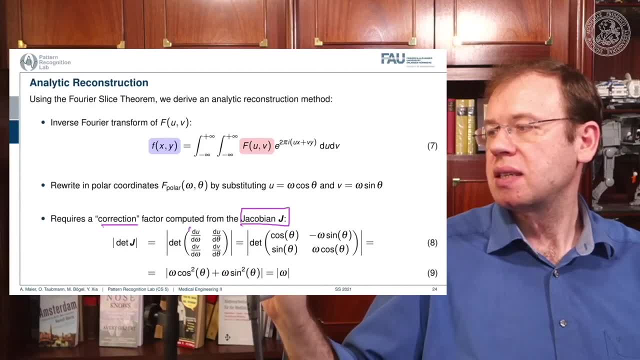 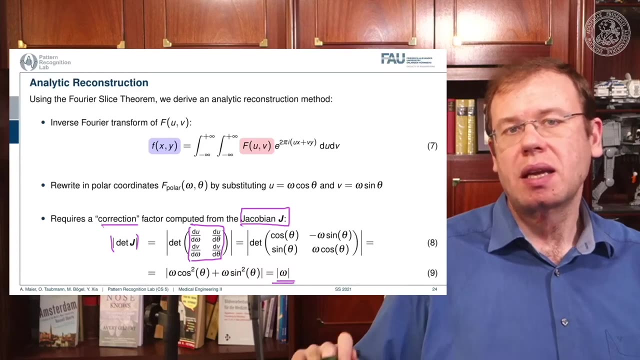 jacobian matrix, and the jacobian matrix is the derivative with respect to the different variables. and then you take the determinant of this matrix and in our case it boils down to the absolute value of omega. so now we know that we have to multiply, in addition, with the absolute value of omega. 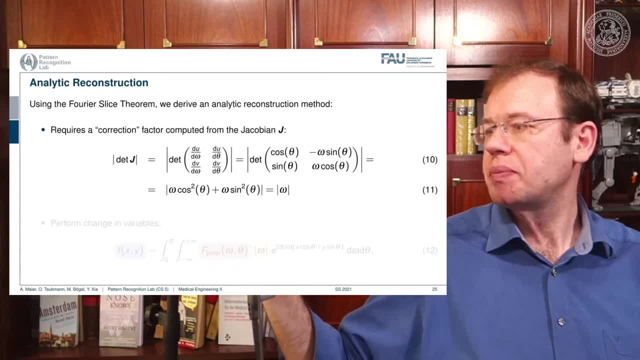 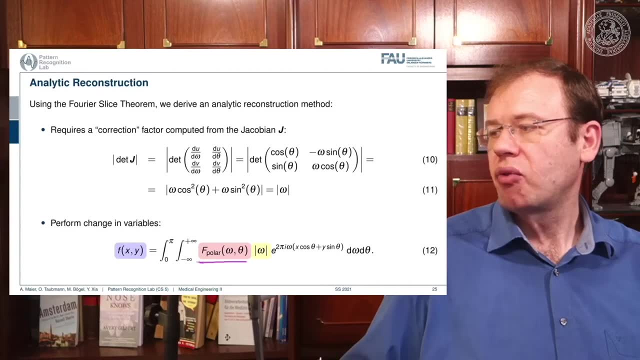 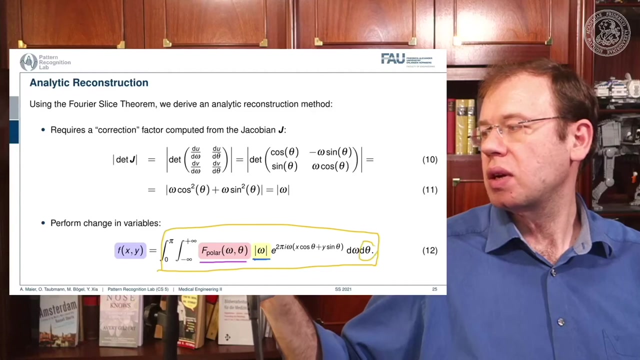 and this means that our fourier transform in the polar coordinate system can simply be expressed as the fourier transform in polar coordinate system and then multiplied with this absolute value of omega, and still the remaining fourier transform here is essentially a fourier transform. differences are now that we integrate over the angle here, which means that we 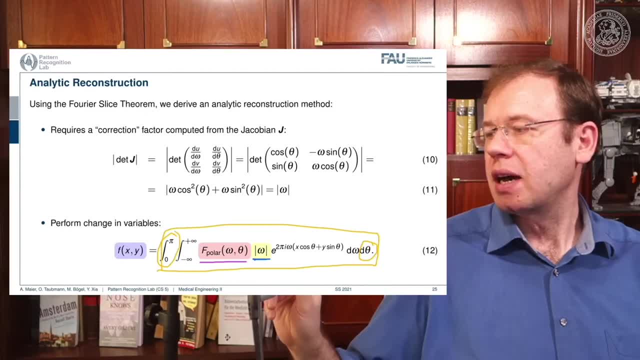 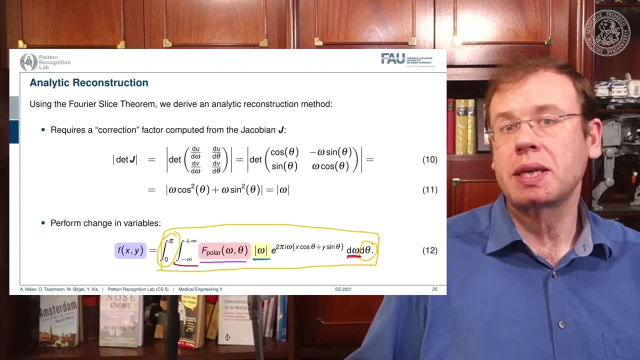 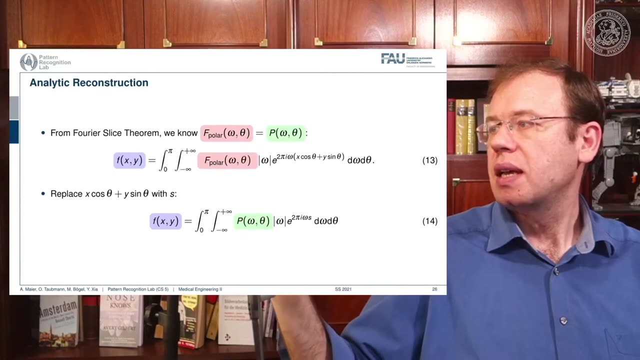 have an integration from zero to pi, and the other variable is still a continuous variable. so this is from minus infinity to plus infinity along the frequency variable, omega. so if we stick to this, then we can now use the fourier slice theorem. so we know that the fourier transform of the projection image is identical. 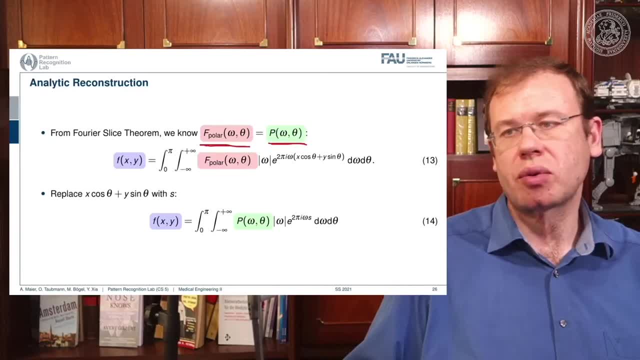 to the polar version of our 2d fourier transform, so we simply replace it and we can now do this change here. the two are identical and now we have a reconstruction formula that has essentially the projections on the right hand side and the reconstructed image here on the left hand side. 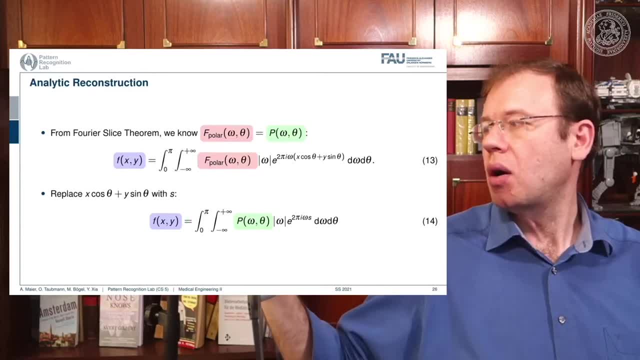 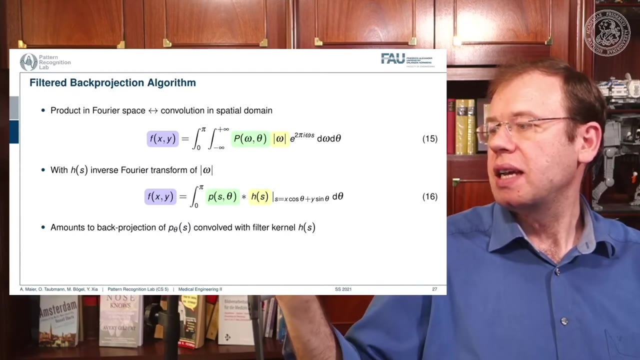 obviously we somehow have to compute the fourier transform of the projection, and there we can also simply take the definition of the fourier transform and plug it in. so you see here that the fourier transform here is actually found in a 1d version. you see this guy here, this: 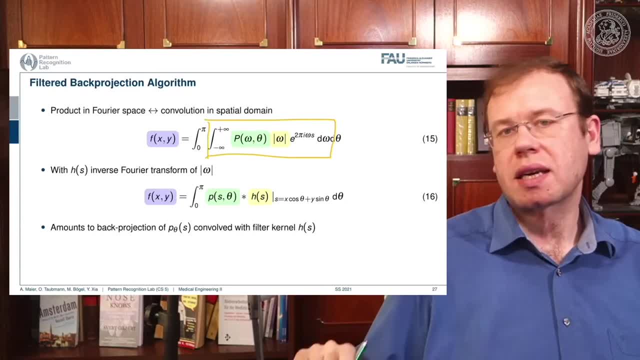 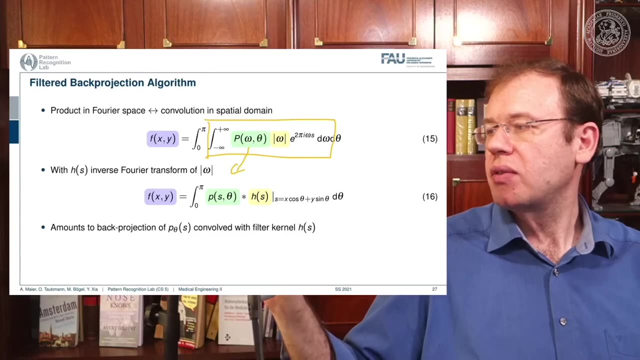 is a 1d fourier transform along exactly the direction in which also our detector is pointing, and this means that we can convert this back into the original domain, so we can save some time. and here you see, then, that we have the fourier transform of the absolute value of omega appearing here, and we also have the original. 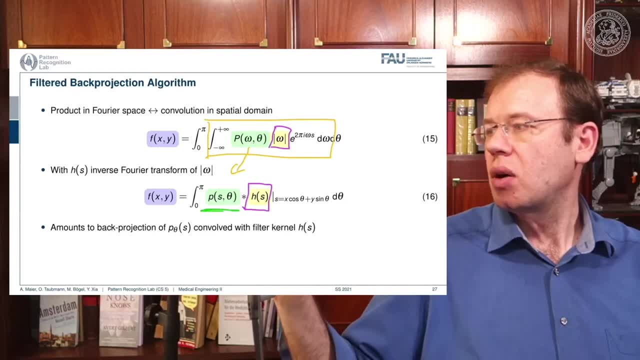 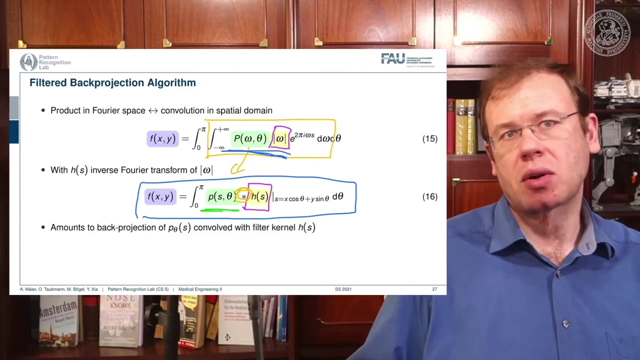 projection data appearing here. so we know that a multiplication in frequency space is a convolution in spatial domain, and this then brings us to the so-called filtered back projection algorithm, the more or less the radon inverse, and this is done by filtering with an appropriate kernel h of s. 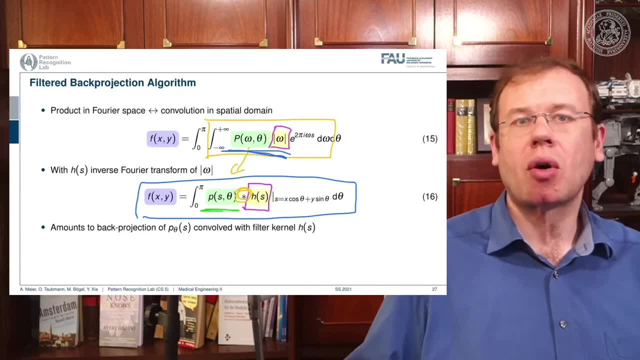 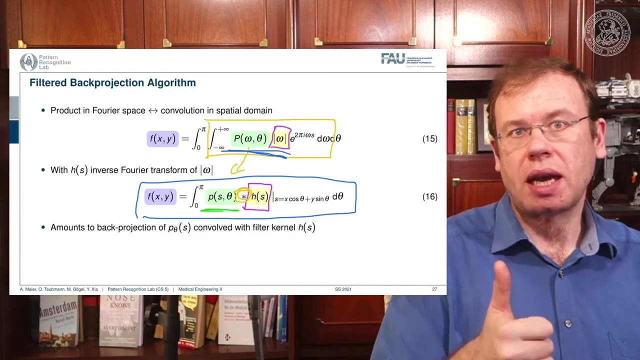 of the projection data and then we just have a sum over all of the projection angles that gives us the reconstructed point. so the steps to actually perform the reconstruction is a filtering and a back projection and with those two steps you can solve the reconstruction problem. and that's cool because the filtering we can do in fourier space. 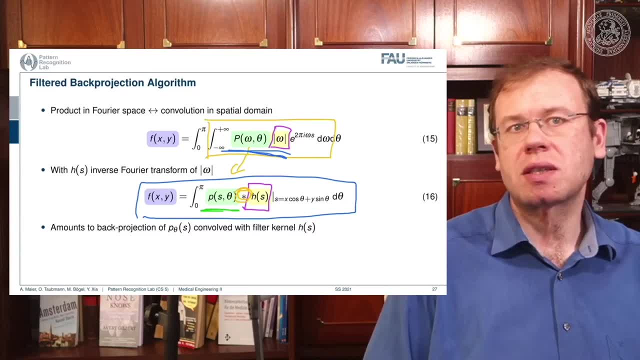 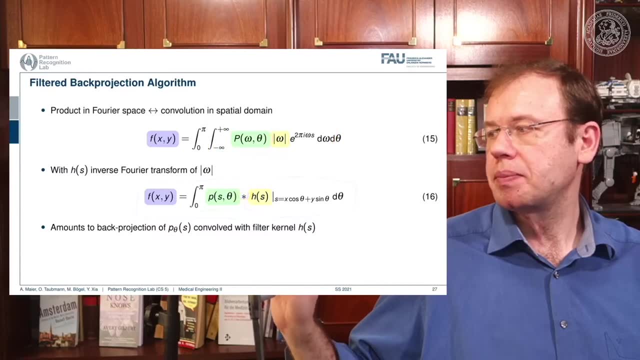 so we have an n log n operation and the back projection is just a single sum, so it has a complexity of n. so this is a very efficient method to solve the reconstruction problem. yeah, so this is the filter that's introduced here. so in order to do that, we have to determine this filter. 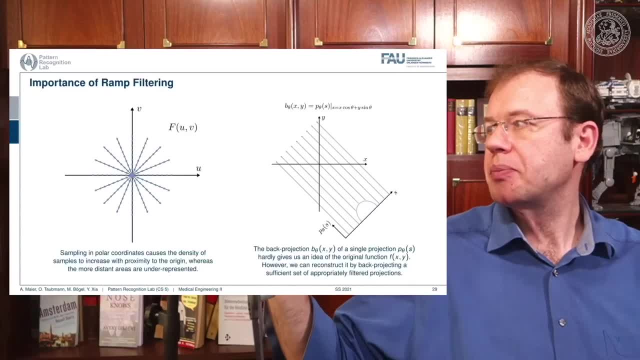 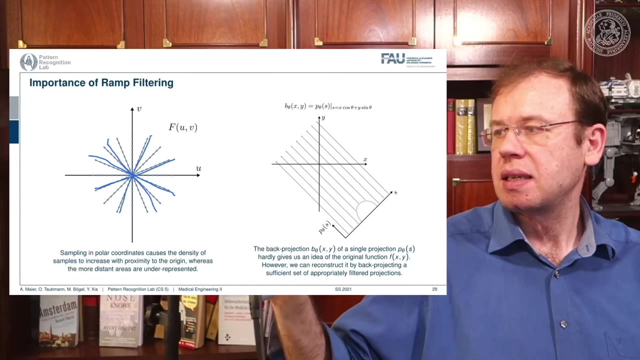 and the filter also has a very nice property. so you can see that we've seen that the absolute value is being used here and we already seen that in the previous video. if we sample on this polar space, you see that the density is much higher in the center, the density of observation. 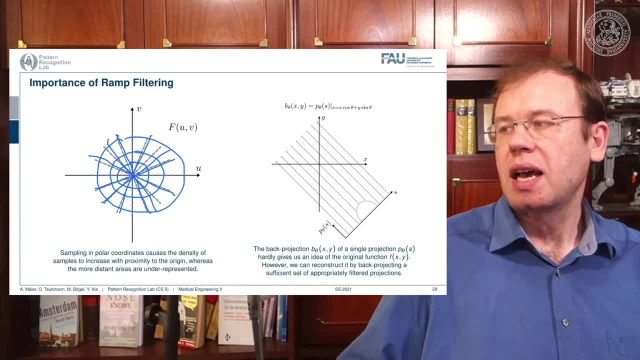 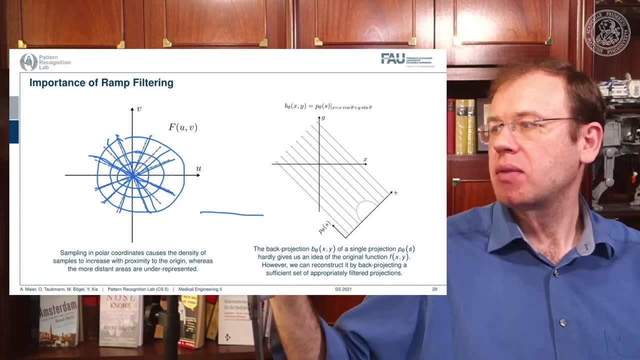 is much higher in the center than in the outskirts, and what we're doing essentially is we take one of those lines here and we multiply it with the absolute value of omega, and the absolute value of omega looks like this and it's it's like a ramp, and you can see that the sampling 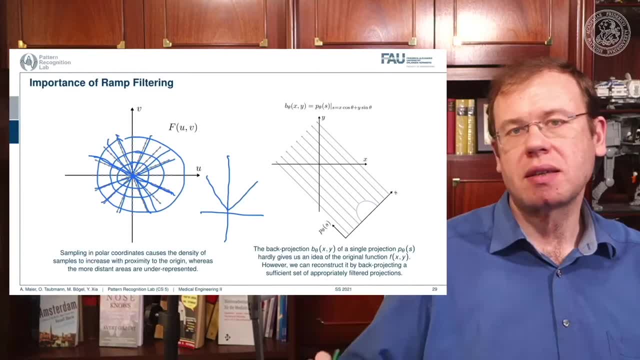 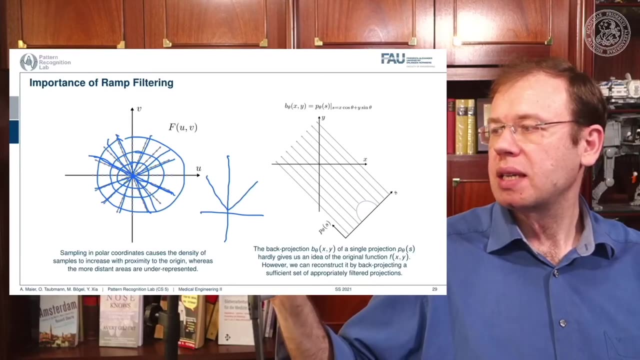 pattern essentially goes down in density towards outside. so we need to ramp up the values on the outside and in the center in a continuous space. actually, in the perfect center, you would infinitely times observe the zero frequency. this is why we are waiting with zero in this ramp. 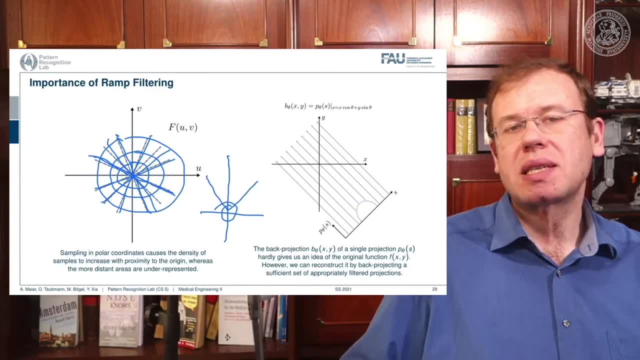 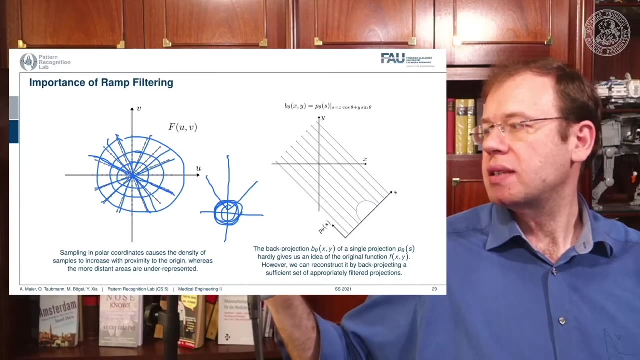 filter in the zero frequency. obviously this is not true if you're going to discrete space and you have to care about this position in the ramp filter a lot when you're actually implementing this in a discrete version. yeah, so this kind of filter is then applied to our projection image you convolve with the 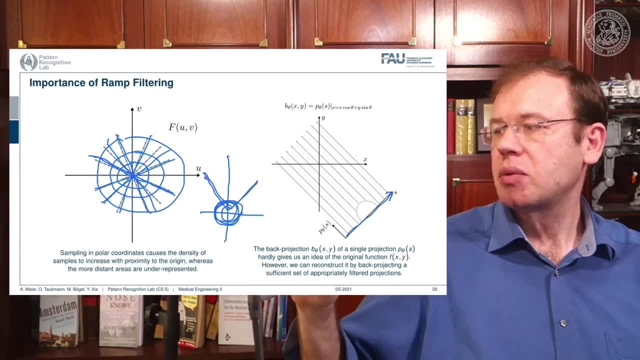 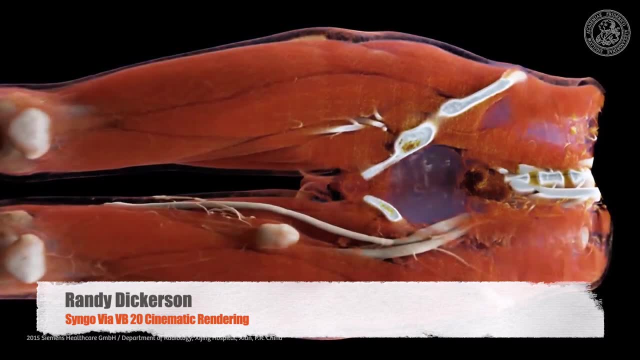 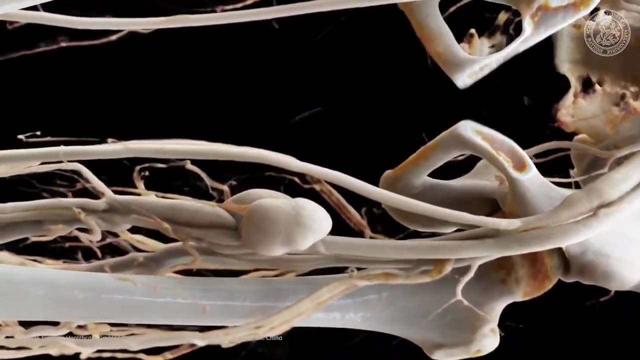 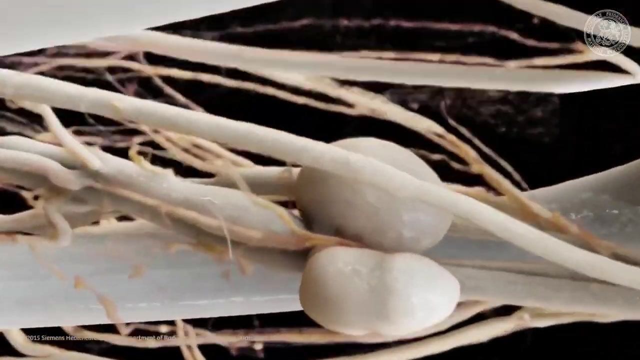 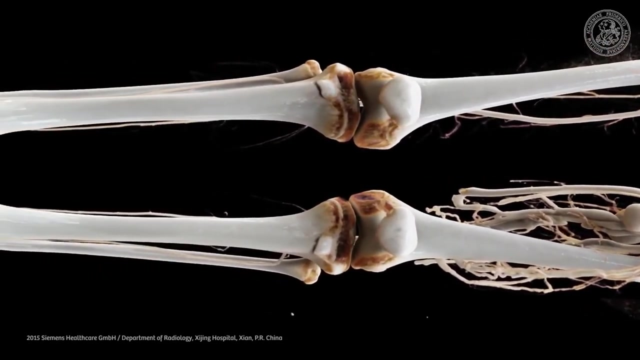 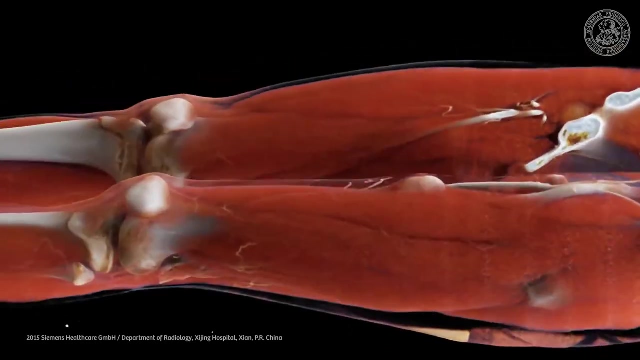 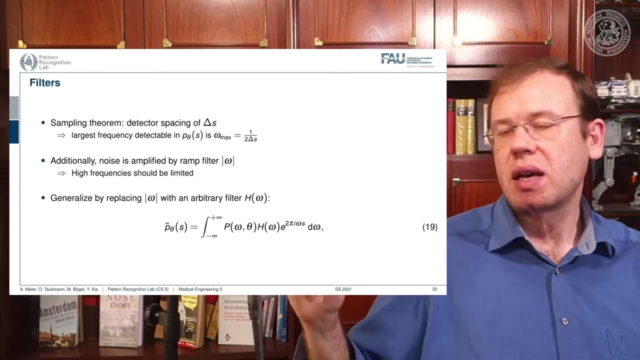 Fourier transform of this ramp filter and then you back project. so that's already how you would reconstruct you. then we still have to talk a bit about this kind of filter and and, and we need to actually cut off certain frequencies because we know that our detector has only finite element sizes. 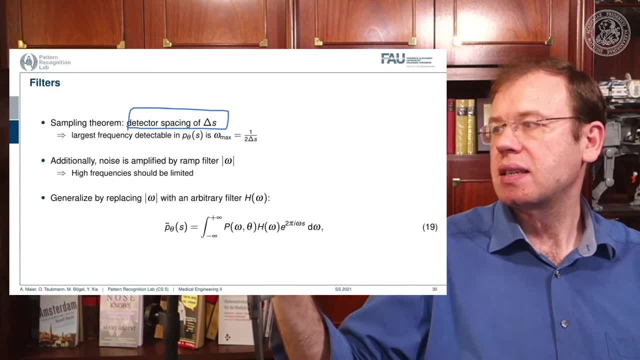 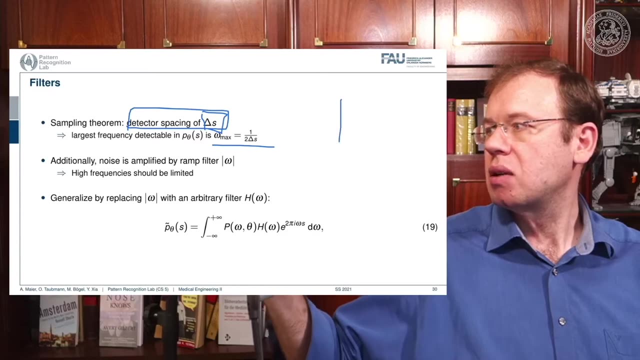 So there's a detector spacing and this has a finite size of delta s. So there is a maximum frequency of 1 over 2 delta s, and this one has to be applied to our RAM filter, which then means that the RAM filter doesn't look like the one that I've drawn previously. 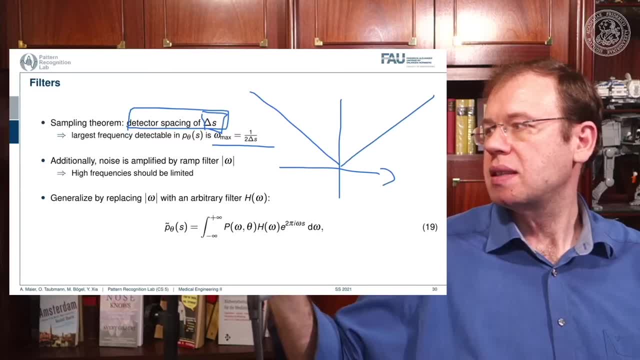 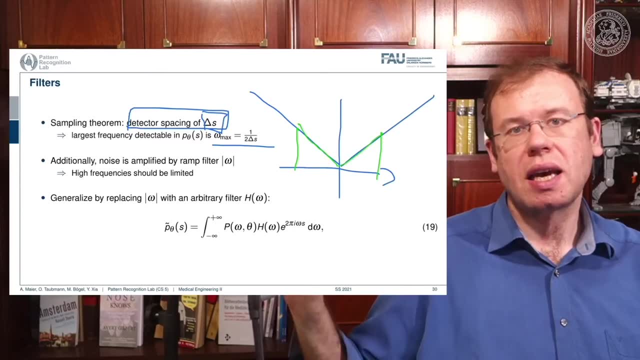 which just goes all the way to infinity, but instead you have a cutoff frequency here and here and the filter that we are actually using has this kind of shape. So then we can actually generalize to an arbitrary filter here, because we may want to incorporate also other kinds of filters. 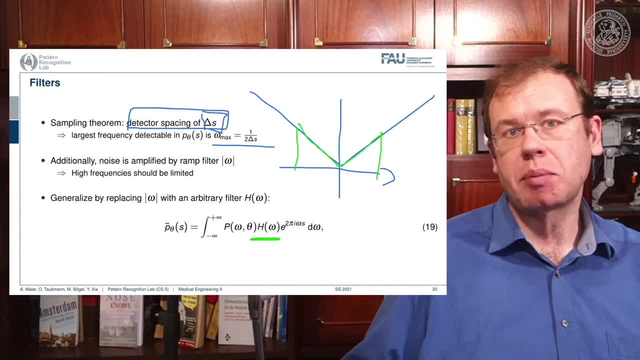 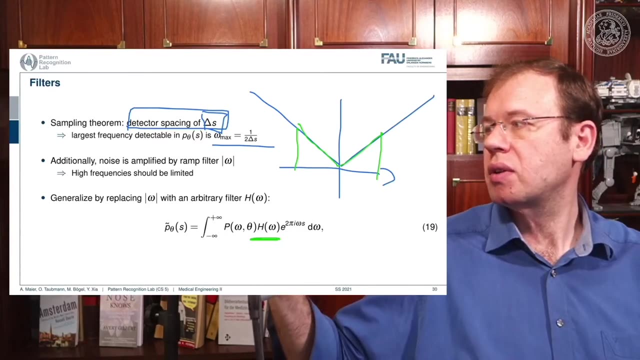 So you see that this is a high pass filter, so it will be very prone to noise, and when we are filtering anyway, we can also incorporate other filtering operations, such as a noise reduction and a smoothing operation, and this then results in alternate filters that have an additional roll off. 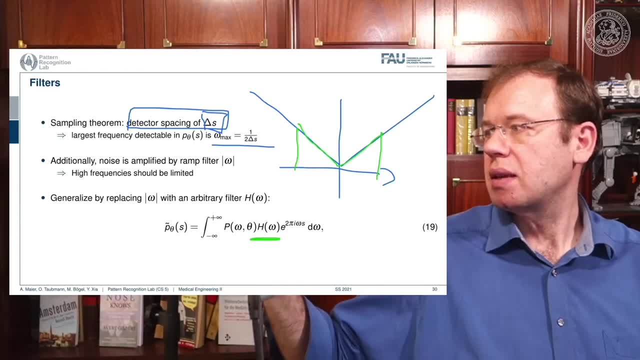 So if you also want to punish high frequencies, you might then get a filter that looks like this one here. So you have a rolling off towards the end of the Fourier space because you want to punish the high frequencies in order to avoid excessive noise, but you still want to keep the low frequencies. 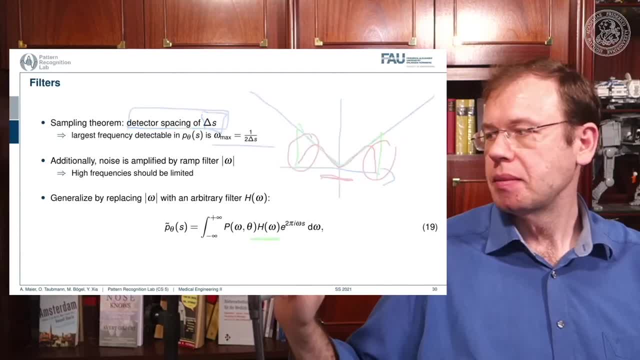 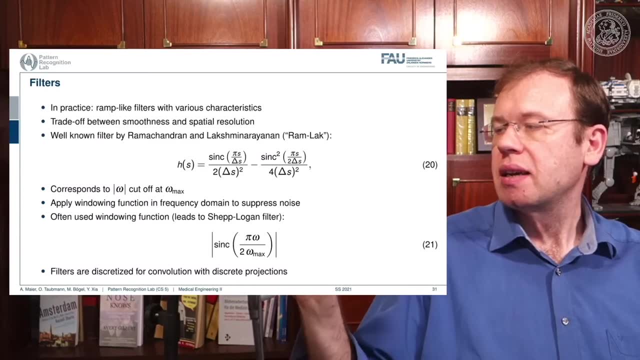 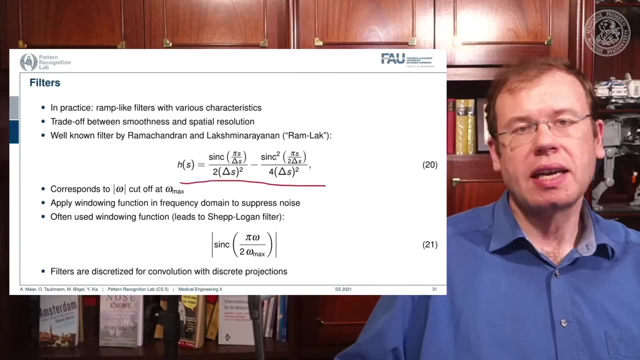 because you want to reconstruct the object correctly. Well, this can then be done also in a mathematical sense. The cutoff version of our RAM filter has a representation in the spatial domain that you find here with this equation. We are not deriving it here. 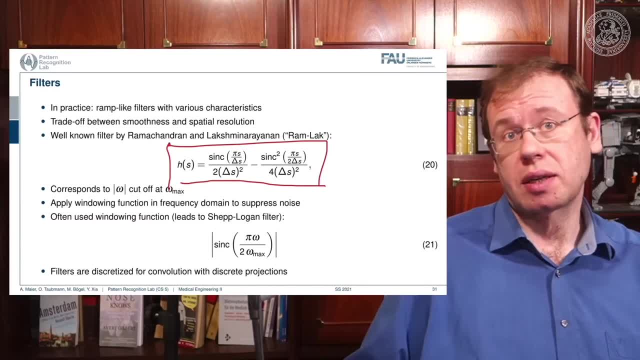 You can look into the textbook. We derived it actually. there. There is a very elegant solution that allows you to derive this in only three or four steps, So that is actually quite efficient, And often times this is then also weighted with one of those cutoff filters. 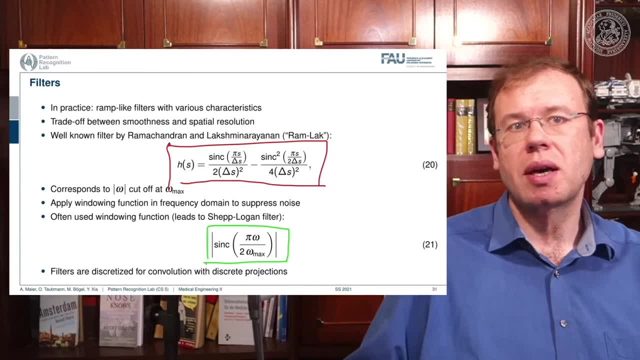 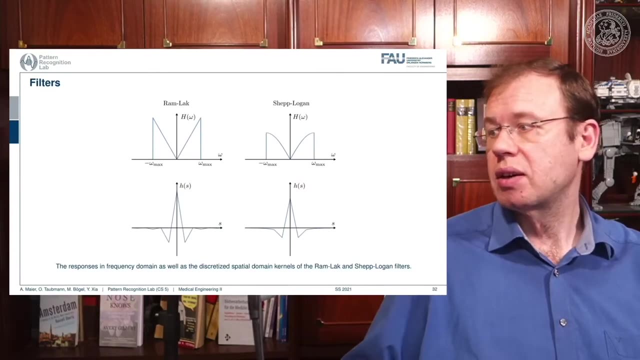 which is essentially a sink that is on top, multiplied into the signal. This then leads to the so called Cheplogan filter, which is similar to what I have just shown to you, And I also have graphs in case you don't want to follow my actual drawings here. 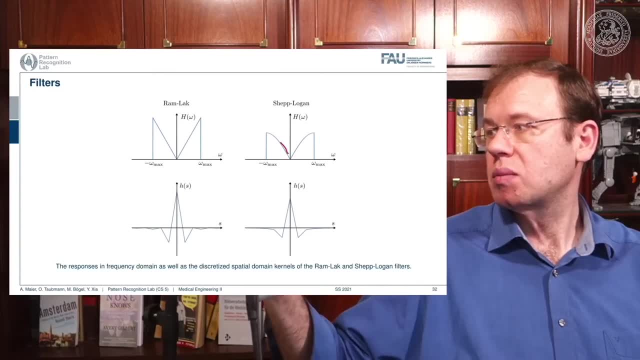 So you see that in the previous version I had a roll off that was much stronger, that was going down here and here And this is actually, I think, the cosine filter that I am drawing here in red. But you see that we kind of punish the frequencies that are very high. 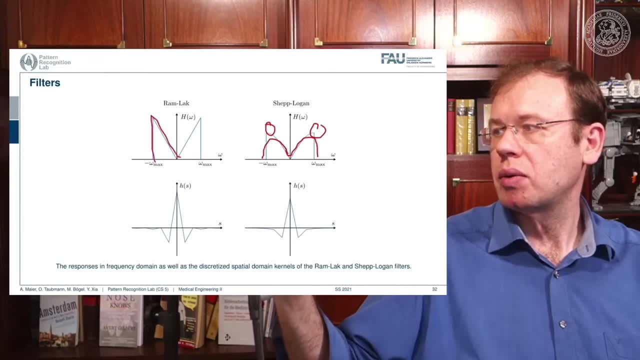 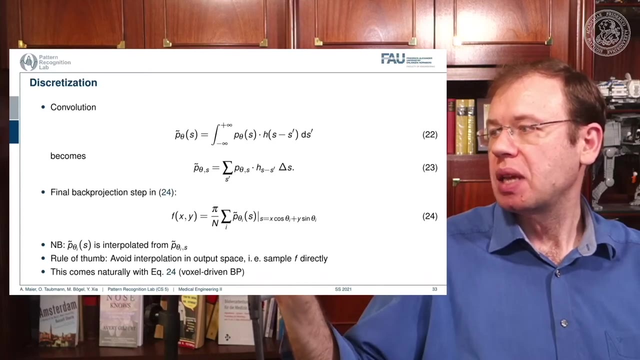 and the original RAM lag goes up all to the very boundary and then just cuts down to zero. So these are different solutions for this filter, And with this filter I can then get the final filtered back projection algorithm. that is a convolution. Now the convolution is actually. 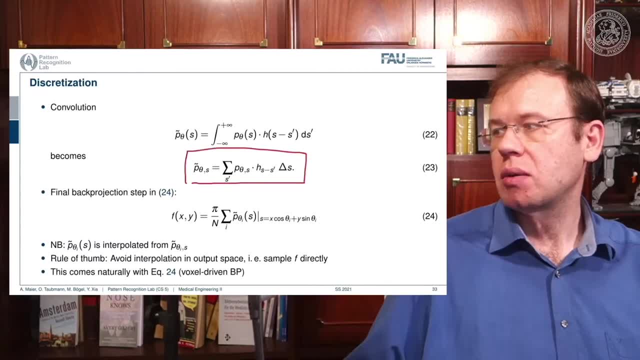 on a discrete projection. This is what we are actually computing. And now you see the integral. in discrete space they just become sums. So it is a sum with our actual filter and the projection image. I sum it up and this gives me this filtered projection image. 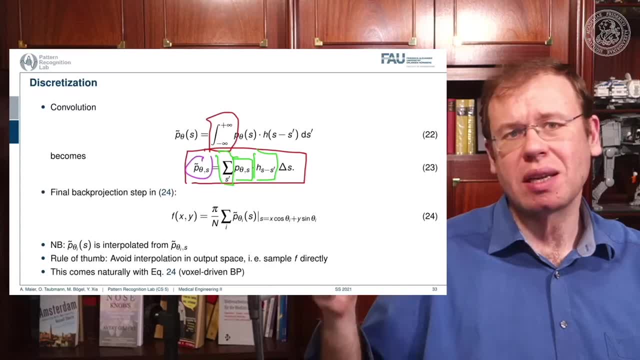 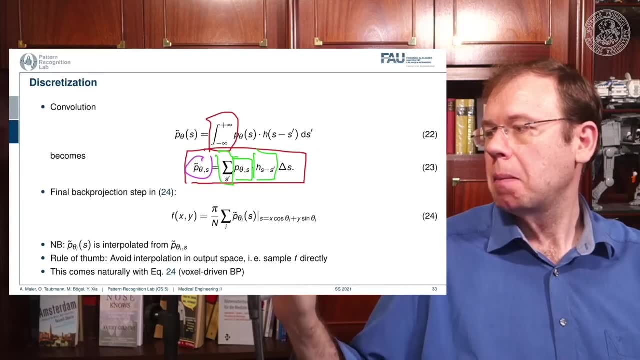 And the filtered projection image is then without any further ado. we don't have to go to Fourier space anymore because we have seen it essentially cancels out. We immediately plug it in to compute our SNISE image, and this is done by the so called back projection. 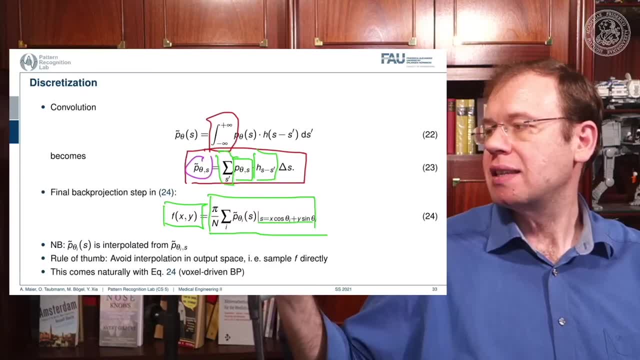 And what is happening here is that I am computing this S essentially as the footprint onto the projection. So if you have your image here, so this is what you want to reconstruct. this is our f the position, and now what I do is I am essentially projecting this. 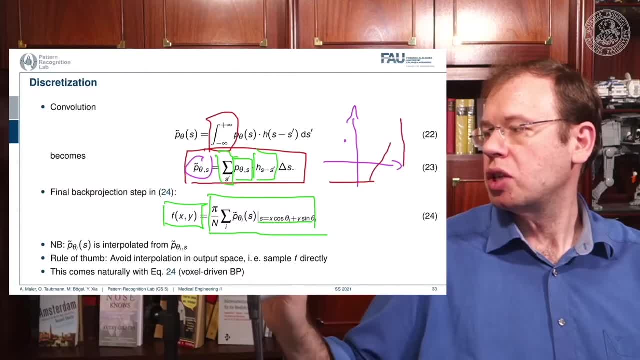 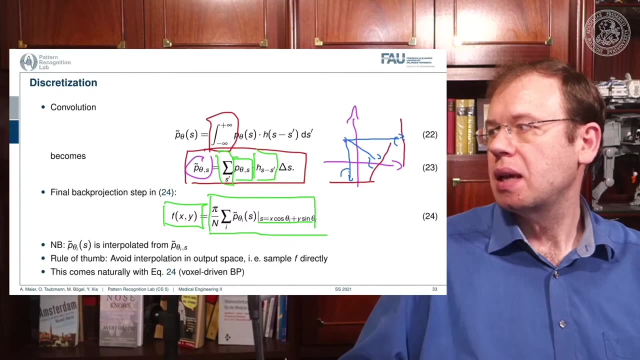 in a parallel manner on all of our projectors and this then gives me the element here, the element here and the element here. So these are all 90 degree angles because we are operating in a parallel beam projection. So this is already the filtered back projection algorithm. 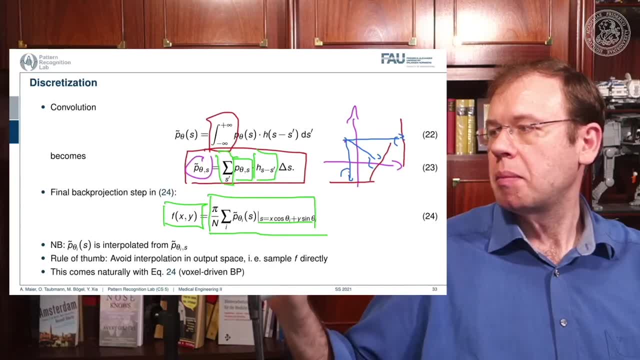 So you implement the filtering, you implement this sum along all of the foot points that you can compute with this kind of equation, and then you get the reconstruction of one point. you iterate over all of the points in the plane and this will give you the entire. 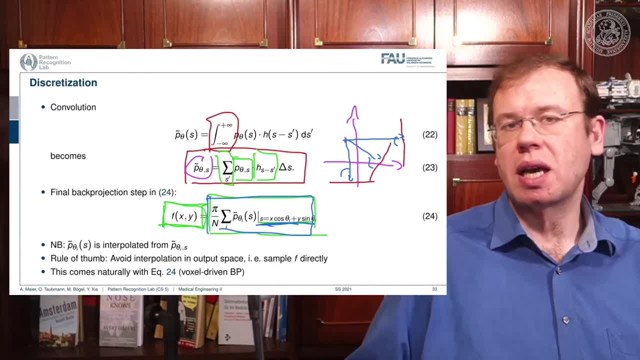 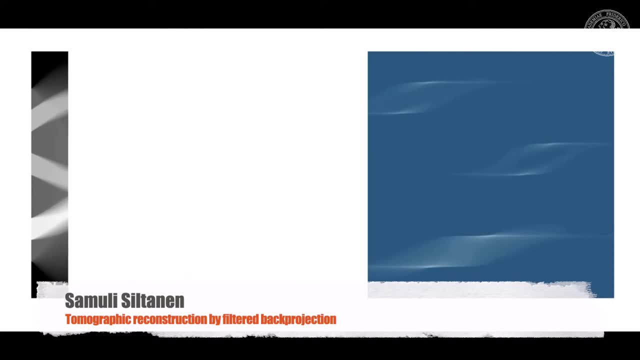 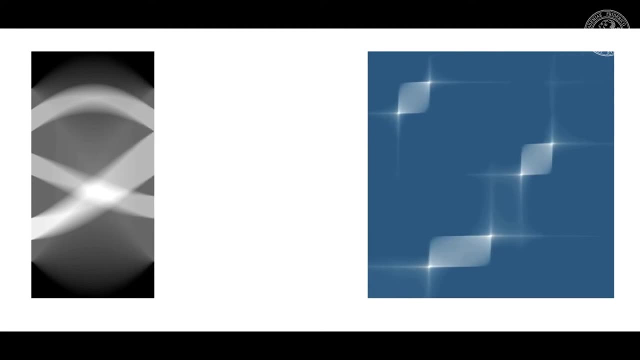 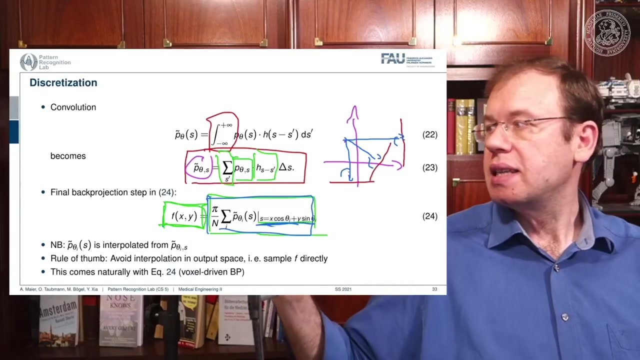 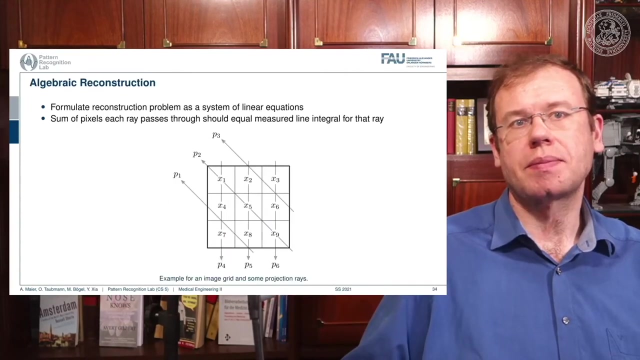 reconstructed image, Very efficient method and still very commonly used in CT reconstruction. There is an alternative to this, and the alternative to this is the so called algebraic reconstruction. And the algebraic reconstruction is essentially the solution that emerges if you discretize first and then solve. 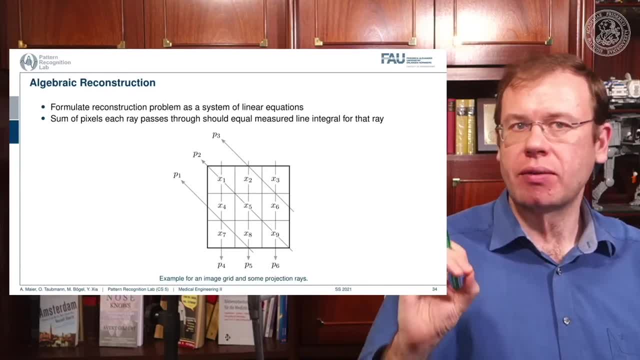 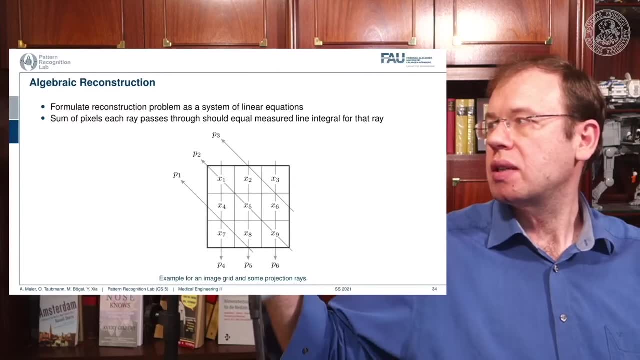 And the filtered back projection is considering everything in continuous domain, and then you discretize towards the very end. Now, if I want to consider the reconstruction problem in a discrete way, I could also describe the CT problem as a set of unknowns and some projection rays. 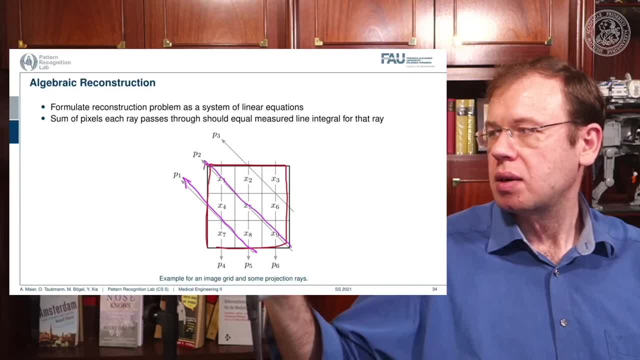 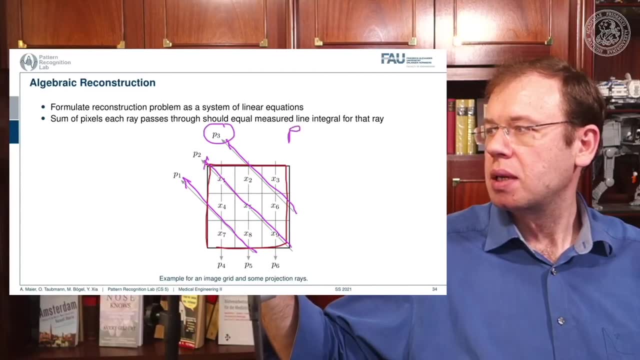 I have my projection rays here, my projection rays here, my projection rays here. This means then that, for example, for this p3, I can simply write up as the sum of x2 plus some weight- let's call it alpha1, and then we also have: 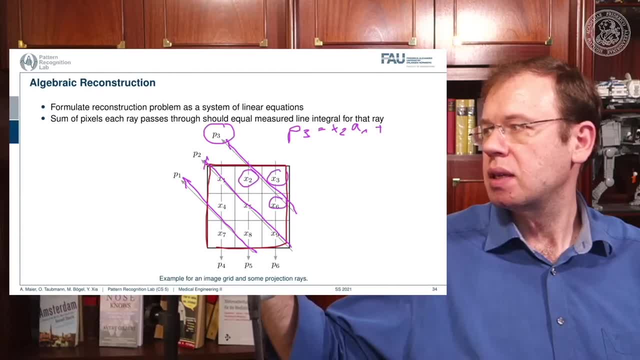 x2 is considered x6 and x3. so we have x3 and some alpha2, and we have x6 multiplied to some, let's say, alpha3.. So what we see is essentially the volume. this is the volume or the slice image, and then I can find: 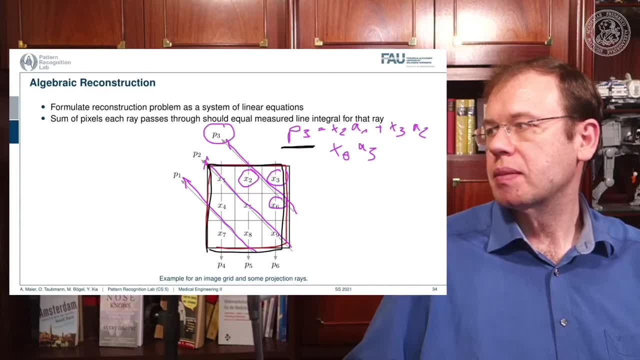 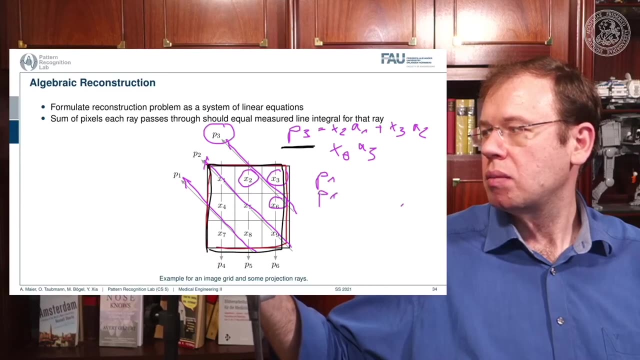 for every projection I can find an equation. So what I can do now is I can write this up as a long kind of vector. so for all our projection rays I can find this in a vector and write this up as p1, p2,. 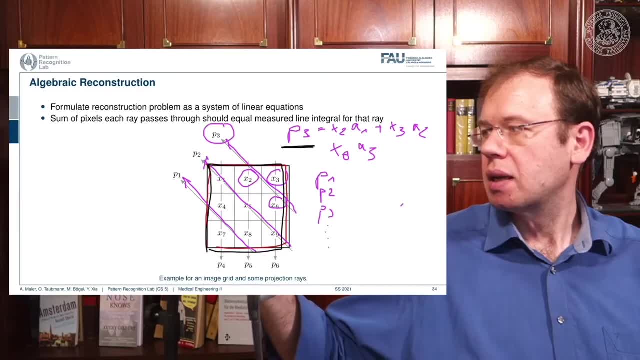 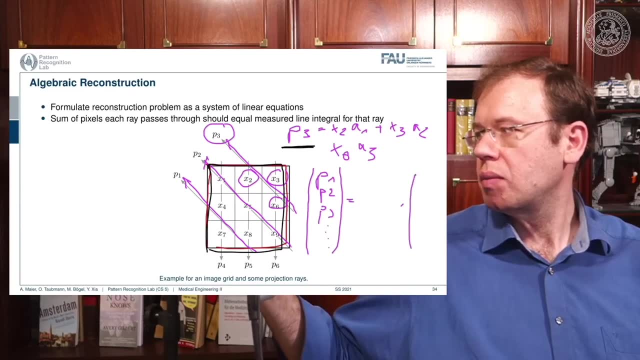 p3 and so on, and I can write this in a long vector and I can also write our entire volume, so x1, x2 and so on. I can also write this in a long vector. and then you see that I essentially have a matrix here and this matrix- 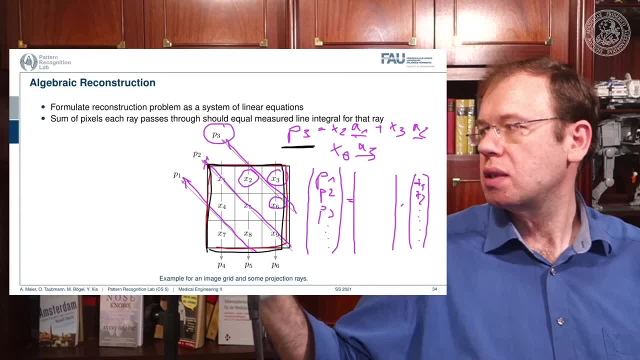 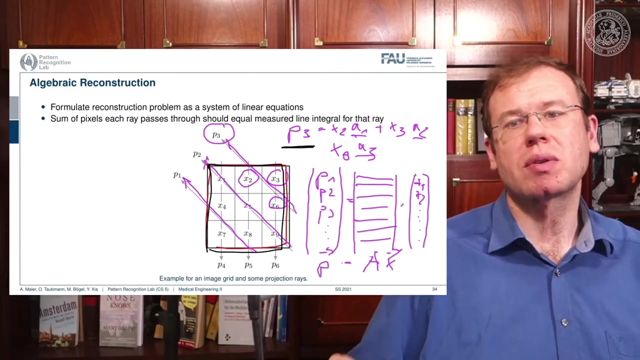 now has nine y's these coefficients. so I can write up this entire reconstruction problem as a vector p that is given as a matrix a times a vector x. that's the entire reconstruction problem from a discrete point of view. so it's a complete matrix equation. just one matrix. 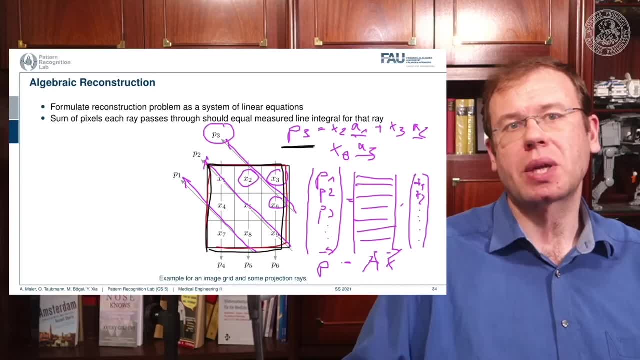 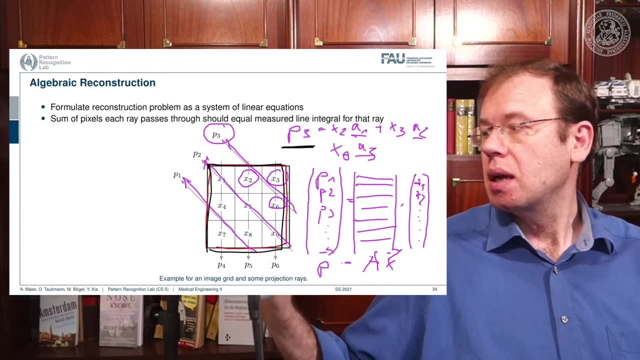 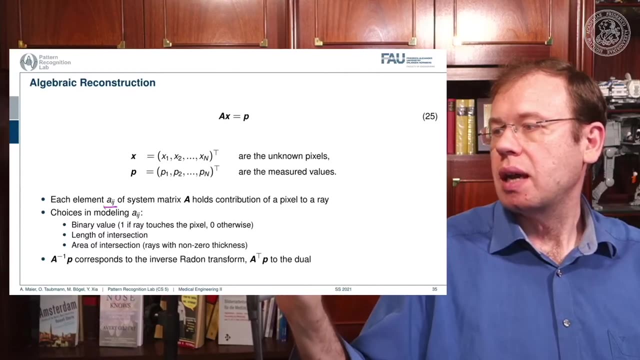 and you can write up the entire forward projection, and then the inverse of this matrix would simply be the solution. well, you see that we can write this now as an equation, and now each element- a, i, j- has essentially the geometric information and it essentially tells you: 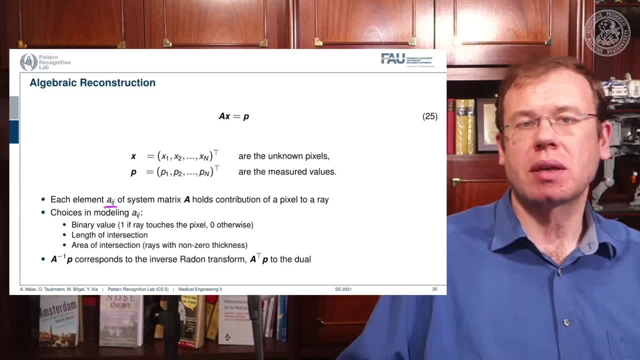 how strongly the voxel is related to this particular point in the projection. so most of the entries of a are actually zero, because if it's not touching the ray, so if the voxel is not touching the ray, it has zero contribution to that particular pixel. so most entries are zero. 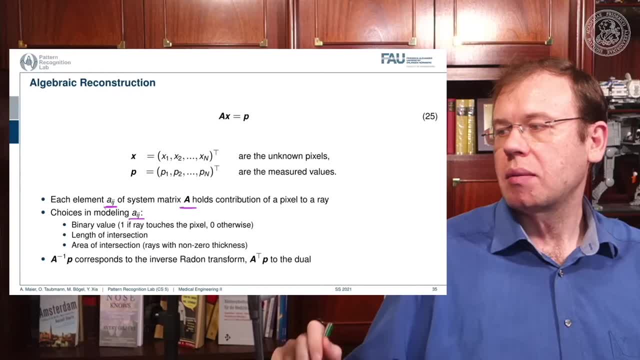 and you can then do different models. so you could say, I can model a, j by a value of one if the ray touches the ray, and zero. otherwise I can compute the length of the intersection, or I could even use the area of intersection to determine those weights. 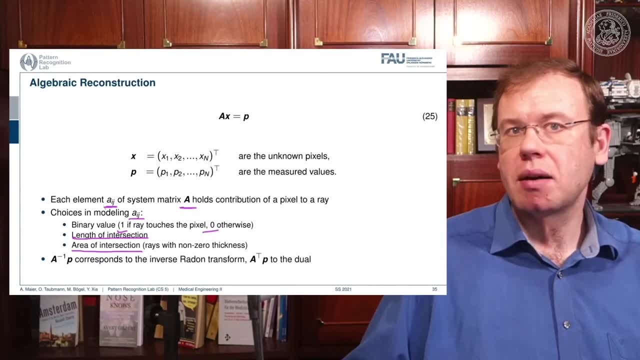 and you see, the more effort I put into modeling this, the more realistic my forward projector gets. but there's many different choices that I can simply model as this matrix A. so now what we want to do is we want to compute A inverse, and this actually is nothing else. 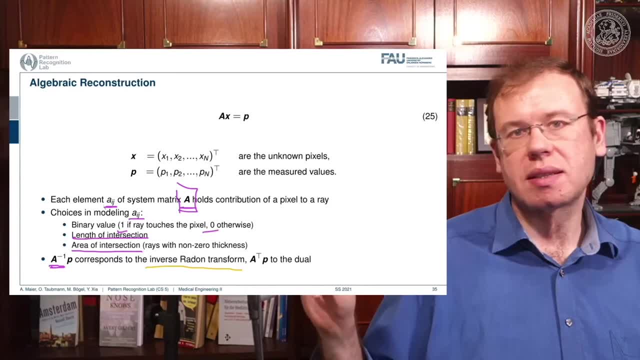 than the Radon inverse that we've seen before. so this is a very interesting observation, but we can also solve it in a discrete way. now, a key problem with this A is that it's really huge. so if you have a volume that is 512 times 512 times 512, 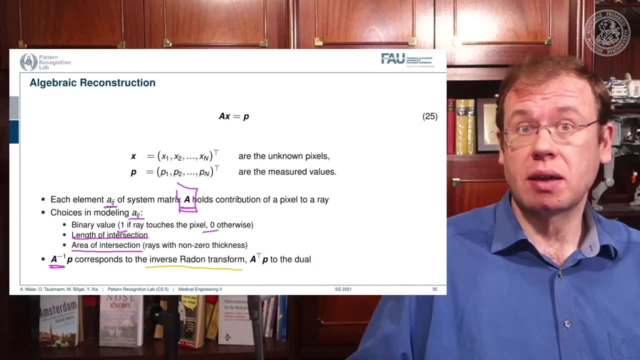 and you have projection images that are 512 by 512 pixels and you have 512 projection images, then you can instantiate a matrix that is 512 to the power 3 times 512 to the power 3, if you want to save this matrix in memory. 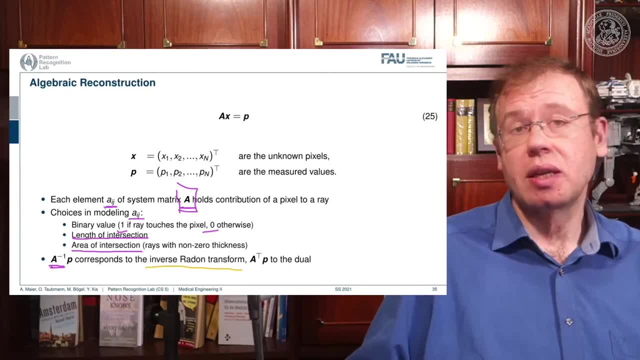 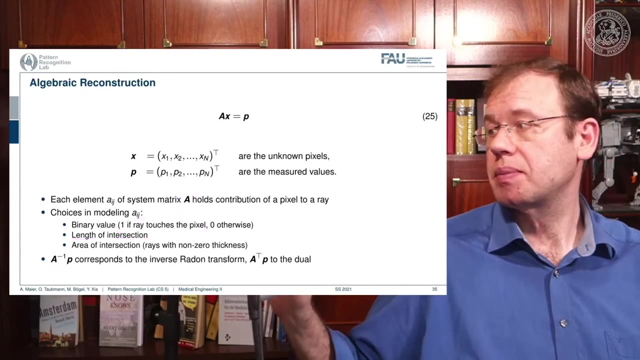 just to store it in memory- just the geometry- you will need 65000 terabytes of memory in floating point precision. so that's not a good way of actually implementing this, and this then gives rise to the so called iterative reconstruction approaches. so this simple solution is not feasible. 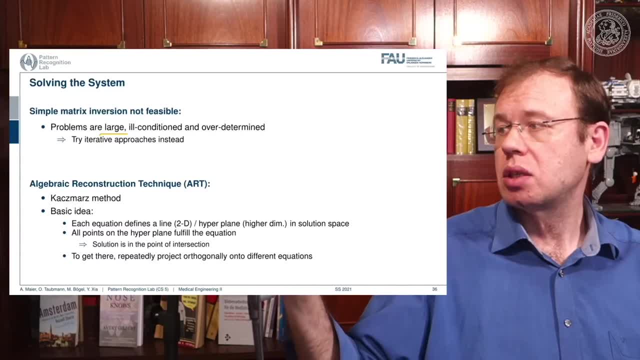 this is really large, it's ill conditioned, it's over determined, it doesn't really work. so let's try to solve it iteratively. and this is where the so called algebraic reconstruction technique, ART, comes into play. it's also called the Katzmarsch method. 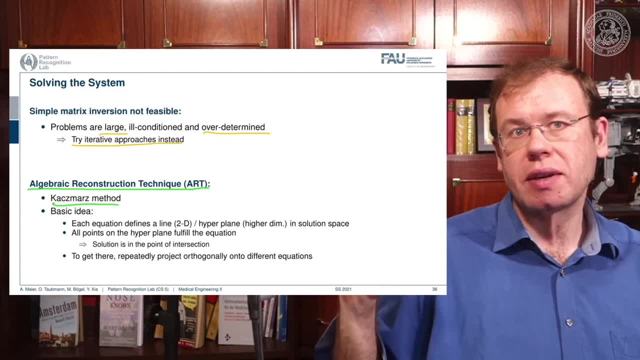 and the basic idea is that you try to iteratively approximate the ideal solution of all the line equations and once you found a new solution for one of the line equations, you project the solution onto the next line, so we have essentially only point and plane intersections in order 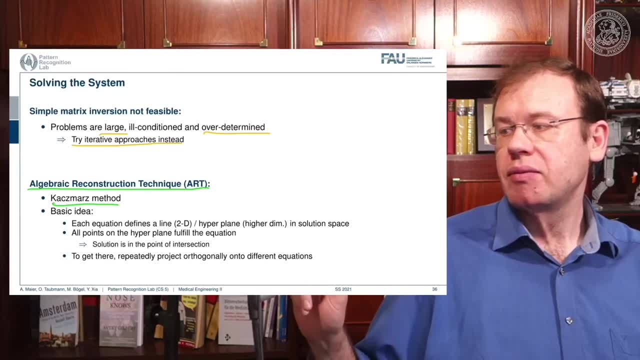 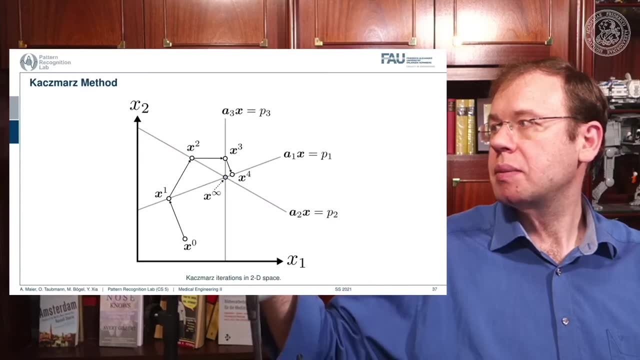 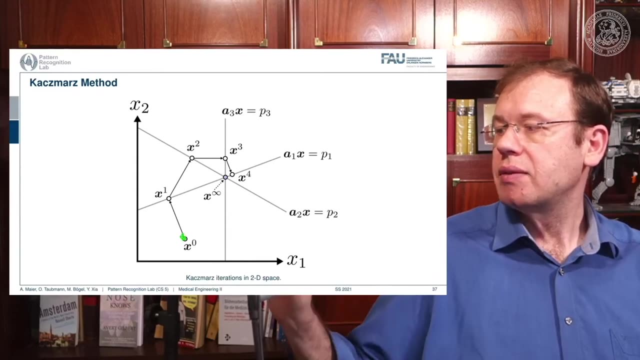 to compute the new update, and we can do that in a successive manner. now, how does this work? well, I have a very nice image here, so you can see that we start with some initial point x0 and then we have a first projection. this is our first projection. 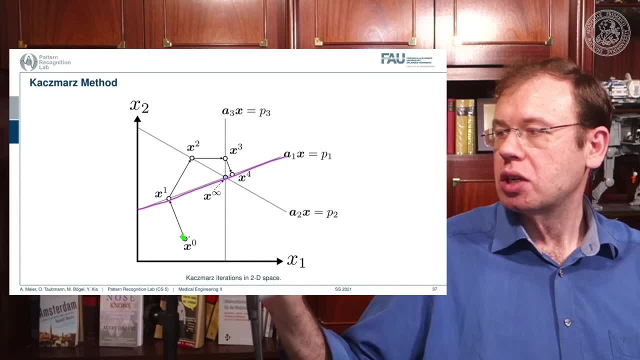 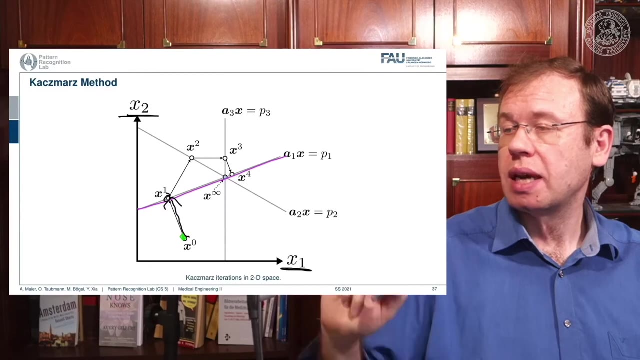 and we now compute a parallel projection from this point onto our first projection and we get an update. let's first have a look at what's actually shown in this space. so you see here that this is the value x1 and this is the value x2. 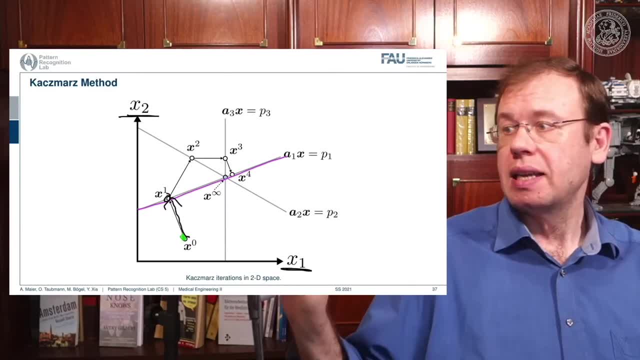 so what I'm showing you here is a volume that only has two unknowns. this has the unknowns x1 and the unknowns x2 and the entire space, so this is not the projection space. so this is all possible configurations of this volume that you see in this space. 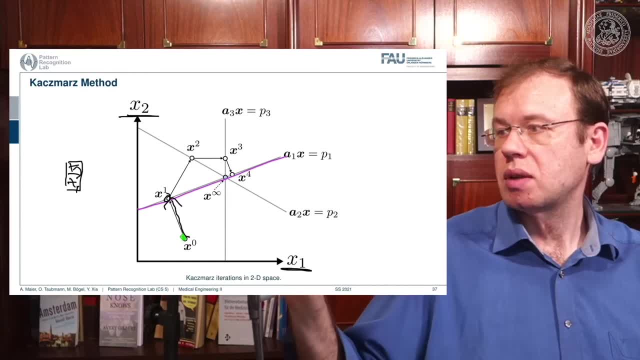 now I start with a random initialization. so you start with some x0, so this could be some initialization here. that brings us here, and then I may have observed some projection p1 here, and this is then the update, such that the observation from this line integral now matches the current. 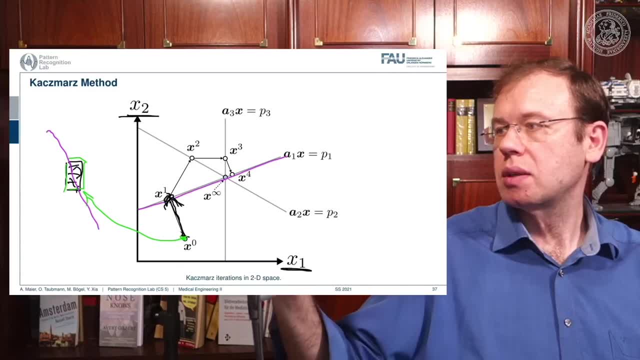 state of the volume. now I can also do another projection. so I'm doing the projection p2, and now p2 is a different linear combination of those two variables, and now I can use this again to create an updated configuration of the volume. and then I have a third. 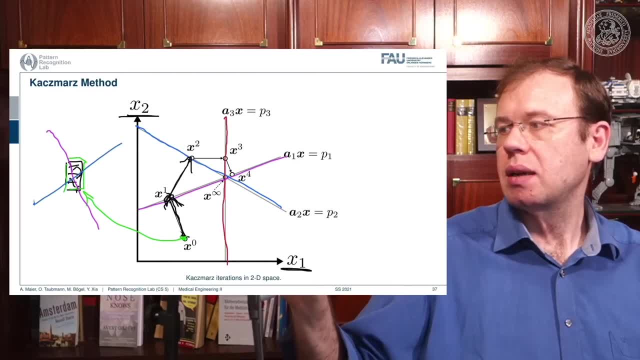 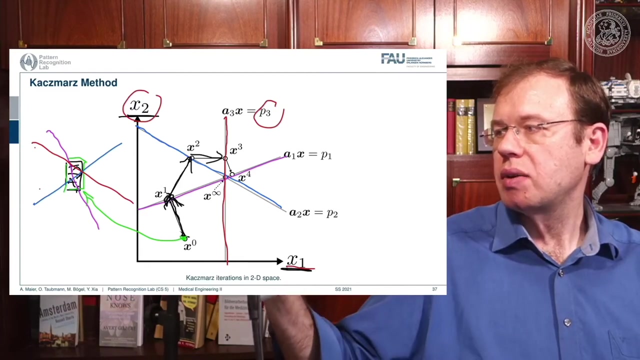 kind of projection that is p3, that runs in this direction for the volume. so you see here that p3 is essentially only associated to the variable x1. now you can see that we can use this information again, that we construct an update and we update again. 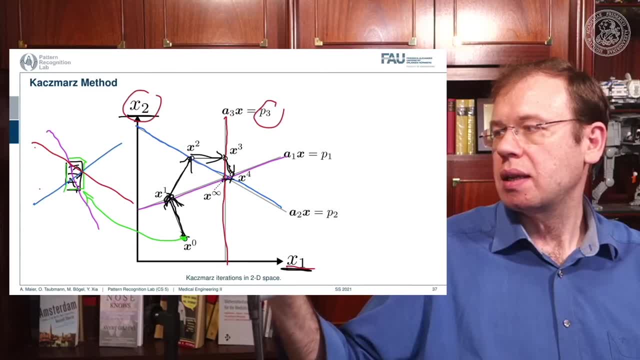 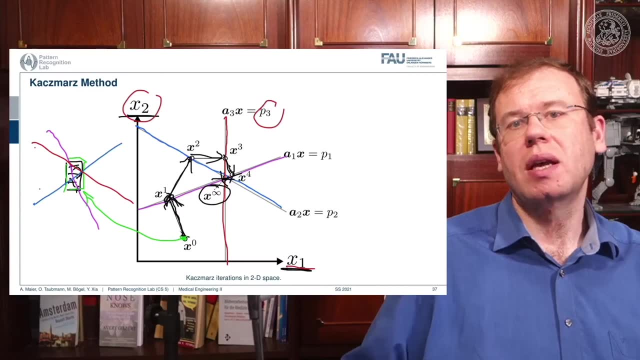 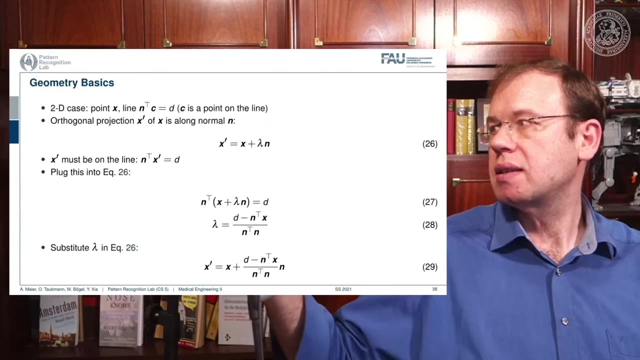 and we update again, and we update again, and then we iterate until convergence and we exactly end up at the intersection of those three lines. so this is the cut-smudge method. now we can also write this up as equations, and you'll figure out that this is. 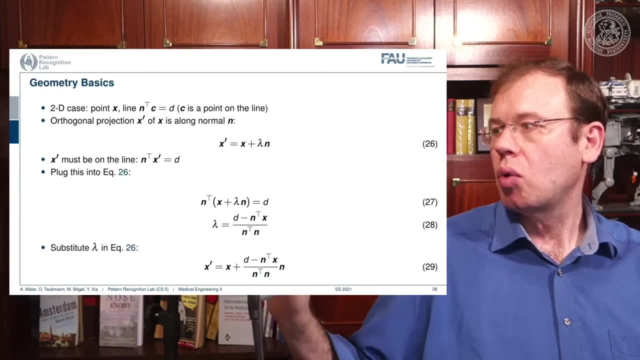 rather easy to construct, because we know that the new observation x' has to be on some projection of the old configuration. you see, this is our original configuration and this is the normal vector of our projection line. so we essentially have to determine this lambda here in order to find 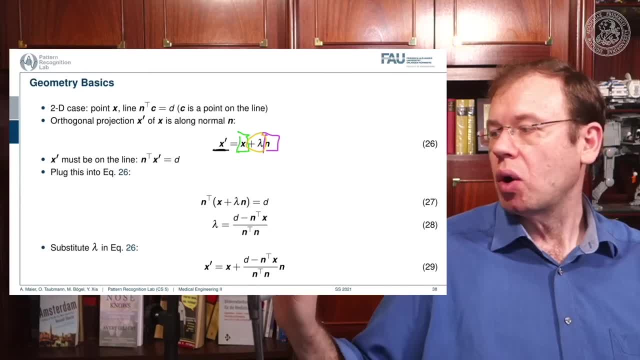 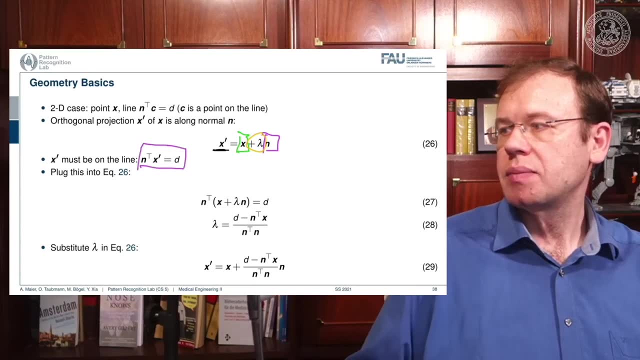 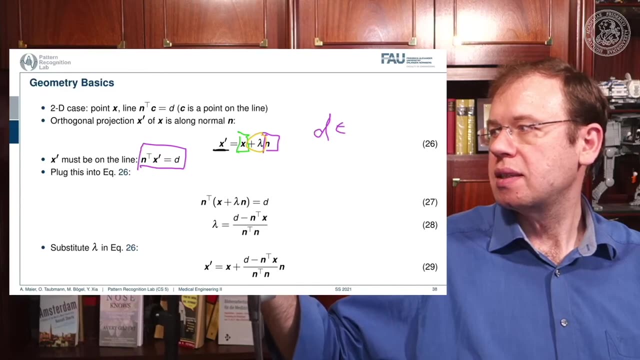 our updated point x' we also know that we have a line equation for our observation, so this is d, but it was called p on the previous slide, so this is d is essentially in the set of p1, p2, p3, so it's one of those three. 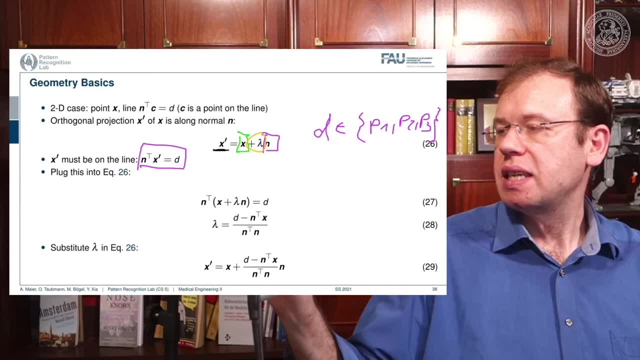 and this is one of those equations, and we see here that the new projection of x' needs to fulfill this equation. that's the orthogonal projection. so now we see that this has actually x' also appearing here, so we can take this definition and plug it in. 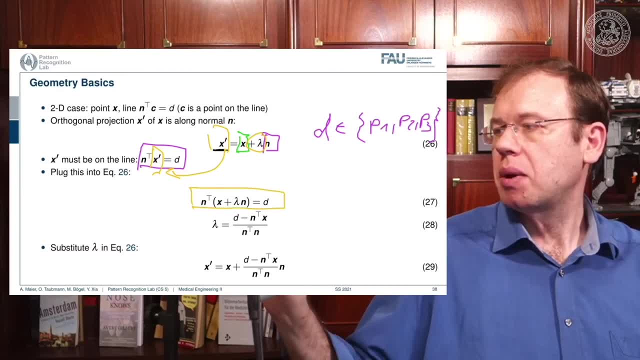 this gives us this new equation. then we can multiply in the n transpose and subtract the n transpose. so here we have the n transpose going in here and going in here, and then we take the left hand term here and subtract it and we take the right hand term. 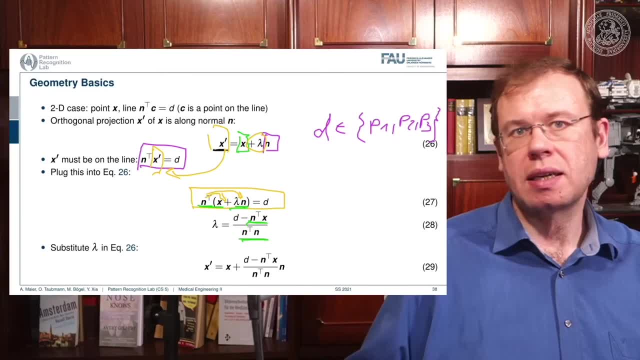 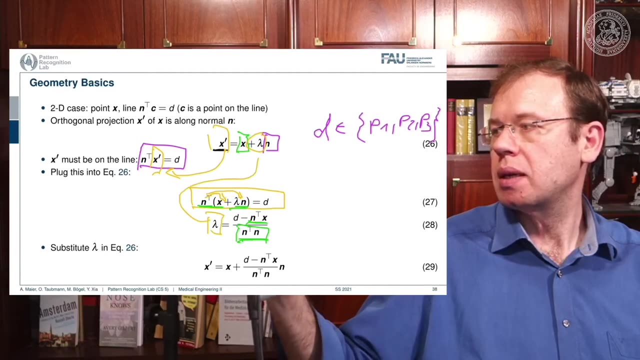 and divide by this: n transpose. n is an inner product between two vectors, and this is just a scalar value. so this is how we can then solve for our lambda, and then we can use lambda and plug it in back in here, and this gives us then the new configuration down here. 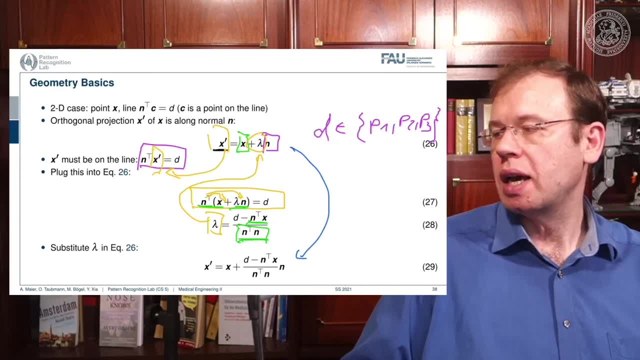 where we have the update, x' equals to x plus. this fraction here times the normal vector. so it's essentially a step length that we have to follow in order to get the intersection with the new point. so this is all just line intersections and orthogonal projections. now 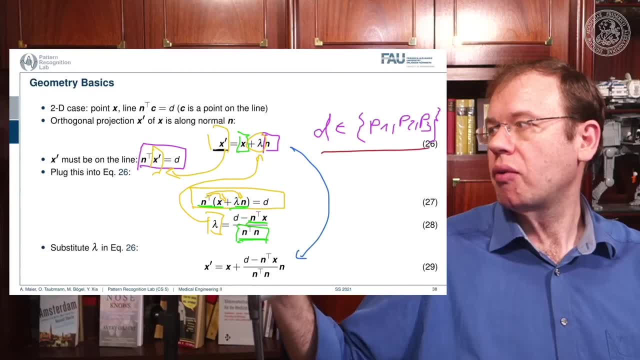 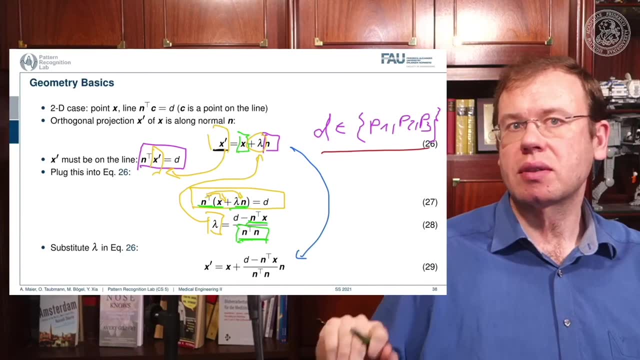 I iterate this over all of our set of the projected pixels and finally I'll find the point of convergence, and this is also a way that allows us to find a solution without having to instantiate the entire huge matrix A that had this many non-zero elements. so this yields then the 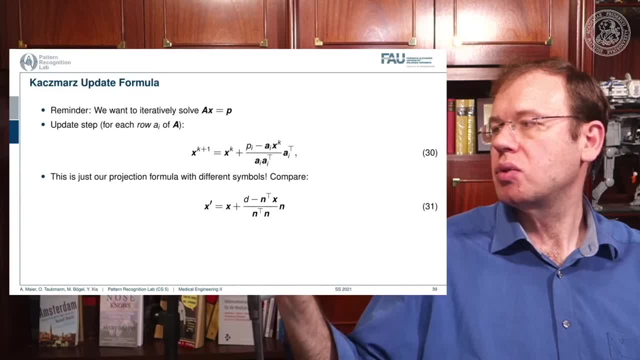 cut-smudge update formula and you do that over the iterations. you see, I now replace this with the iteration index and further you can now see that the end is actually equal to the elements of this matrix. so you see that this is essentially a very similar configuration and we derive 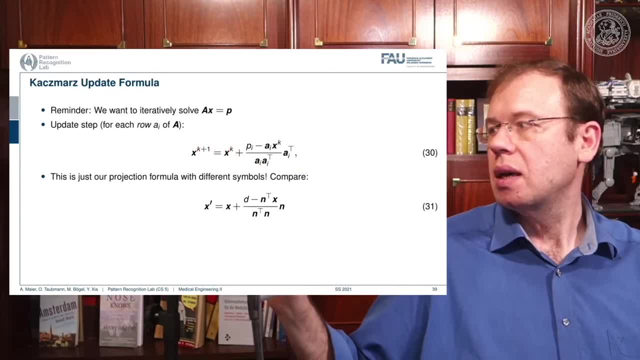 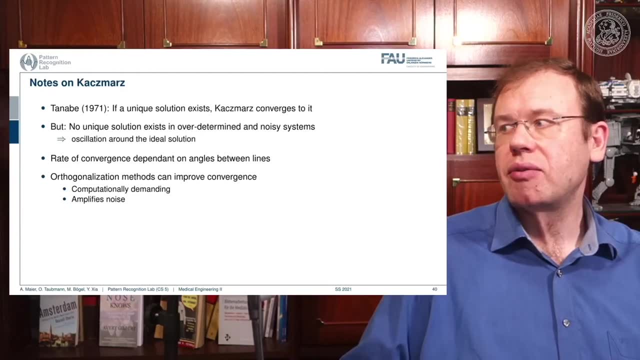 this entirely geometrically good. some notes on the cut-smudge method. there is a unique solution if there is no noise present. so if there is no disturbances present, it will iterate and just find this unique solution. so that's pretty cool, but if there is noise present, 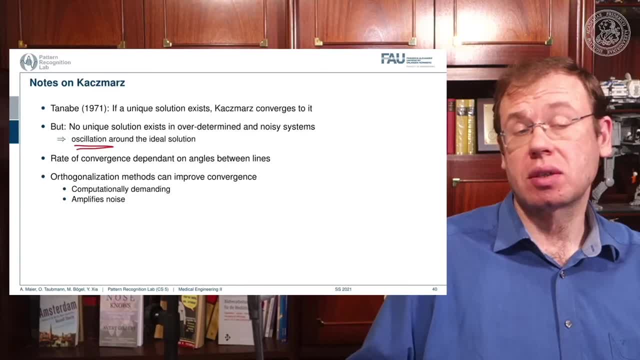 then there is oscillation. it won't converge in noisy conditions and you have to abort at some point. another thing is that the rate of conversions is dependent on the angle between the lines. and then there is also tricks: how to rearrange the system of equations such that the 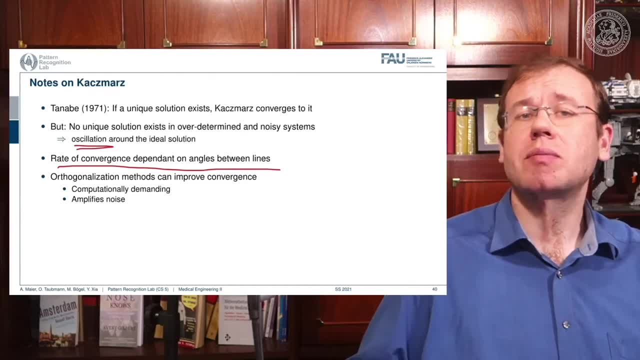 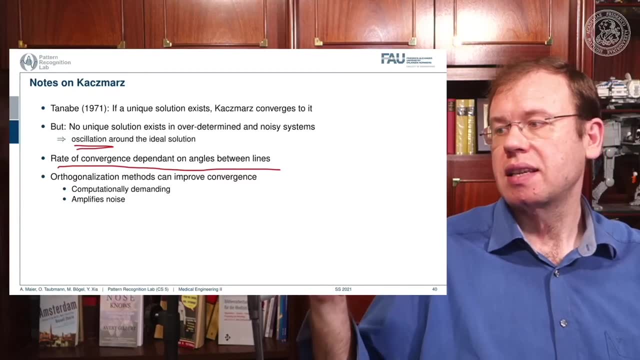 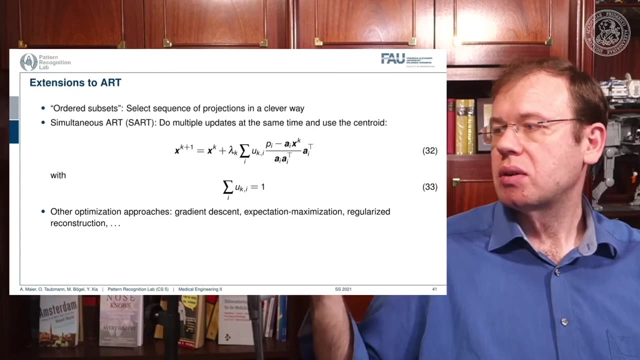 matrix lines essentially are orthogonal, and this brings up quite a bit of convergence speed. if you manipulate the system of equations- and this is some kind of trick that can be used to solve it more quickly- this can then also be constructed into an algorithm that is called the simultaneous ART. 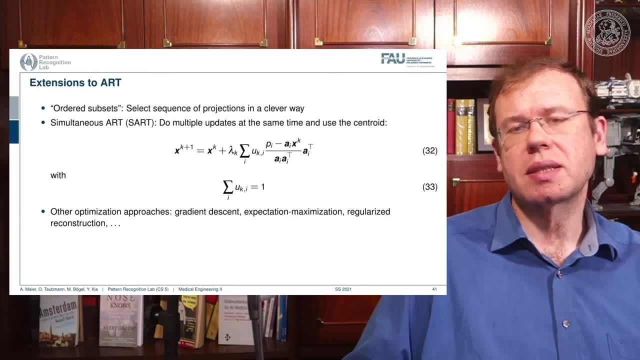 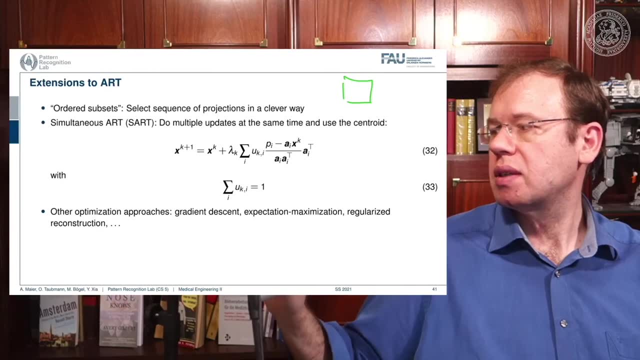 and there is also variance: the ordered subsets. so ordered subsets is essentially skipping over projections. so let's say you have your acquisition plane and then you have projections 1, 2, 3, 4. so this is 1, 2, 3, 4. then what you would like to do is: 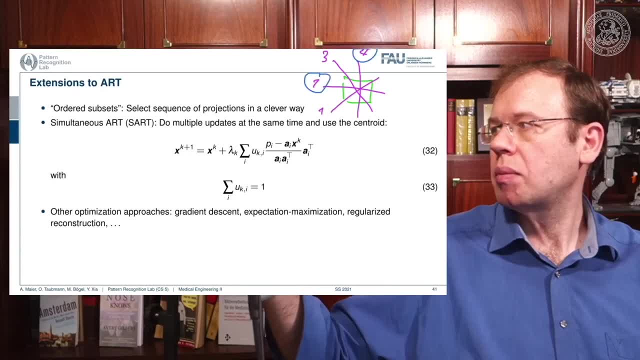 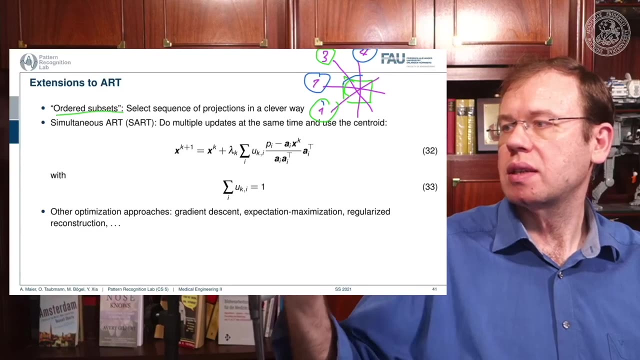 you want to use 2 and 4 because they are orthogonal to each other, and then you update in the next steps 1 and 3 because they are orthogonal to each other. so you try to find projections that will help in the speed of convergence. so this is called ordered subsets. 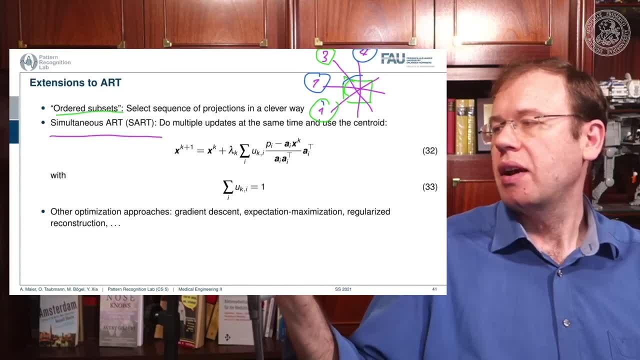 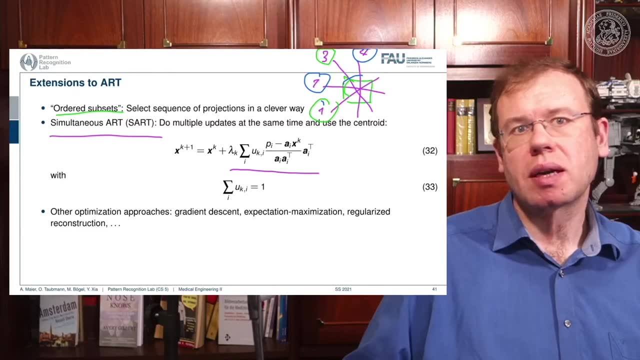 and then there is also the simultaneous ART, where you essentially run up dates over a kind of parallel processing, so you do multiple updates at a time and then average them. so this can also help you with increasing the convergence speed. there is many, many more approaches. we actually have a very nice 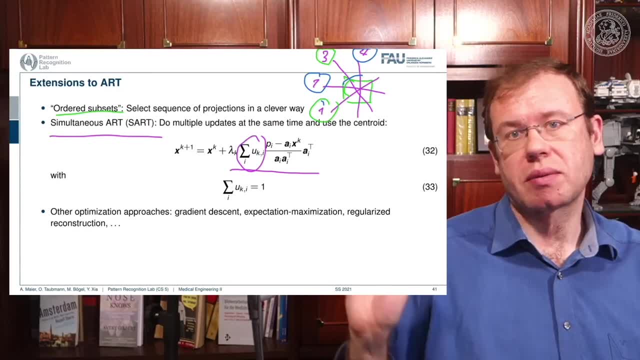 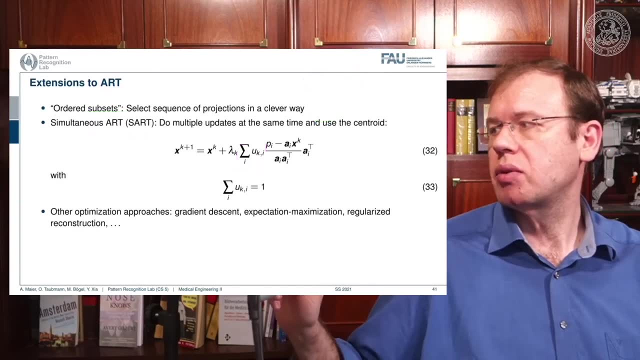 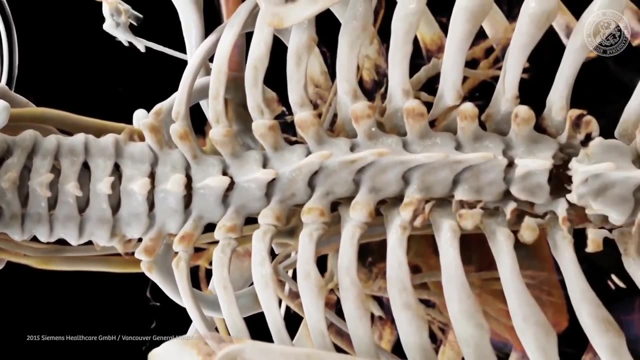 lecture that is called diagnostic medical image processing, where we go into all of these details here and derive the methods and so on. for the time being, I think this is enough about iterative reconstruction, so let's go 1, 2, 3, 4, 5, 6. 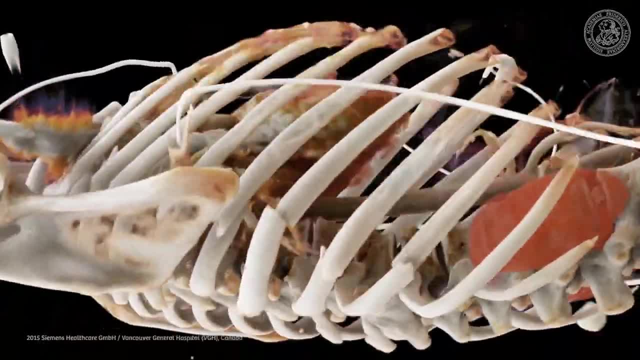 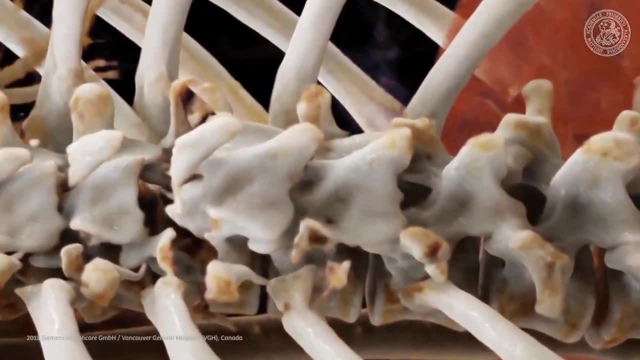 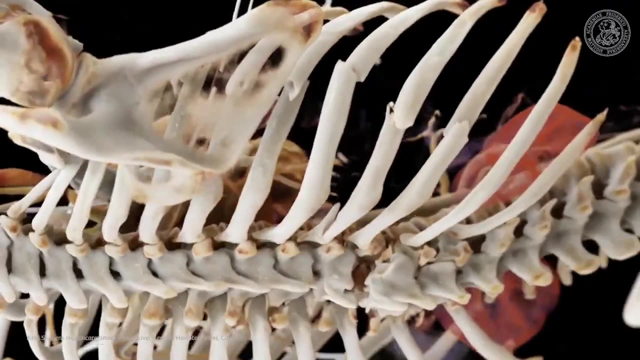 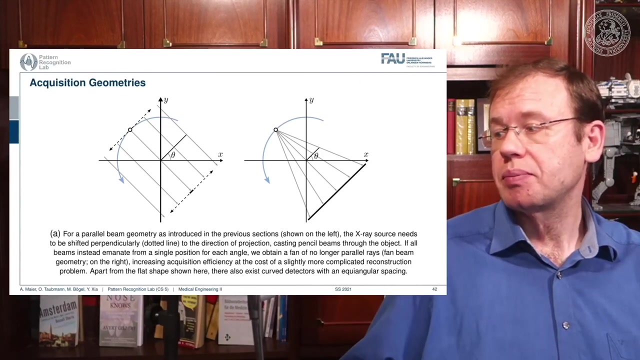 7, 8, 9, 10, 11, 12, 13, 14, 15, 16, 17, 18, 19, 20, 21, 22, 23, 24, 25, 26, 27, 28, 29, 30, 32, 33. 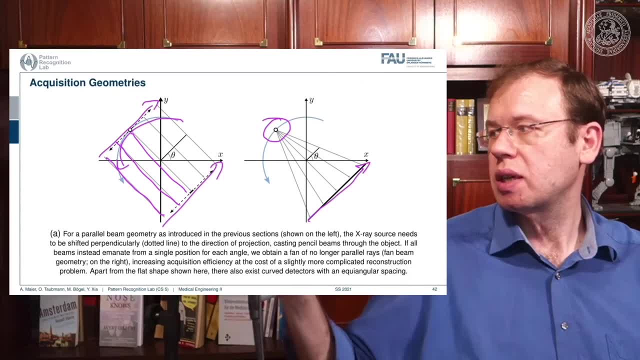 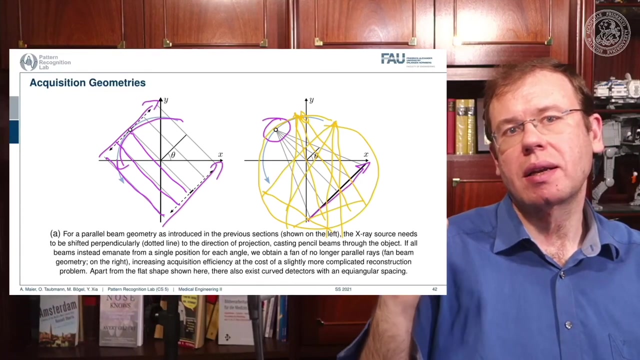 34, 35, 36, 37, 38, 39, 40, 41, 42, 43, 44, 45, 46, 46, 47, 47, 48, 49, 50, 51, 52, 53, 54, 55, 56, 57. 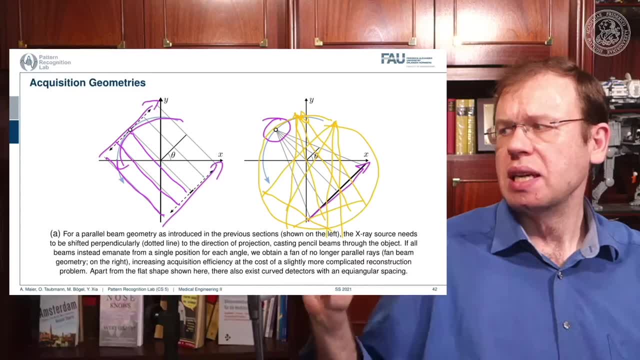 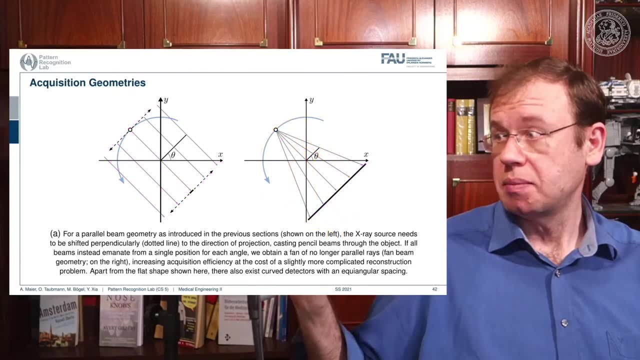 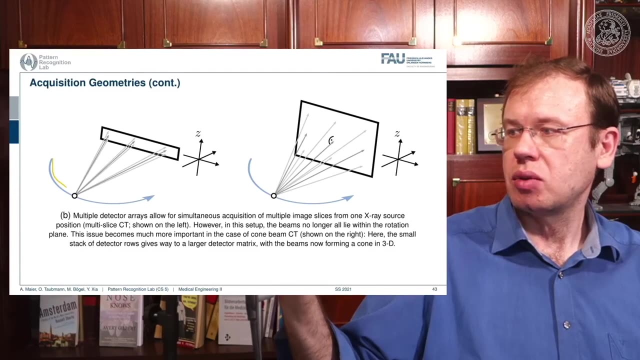 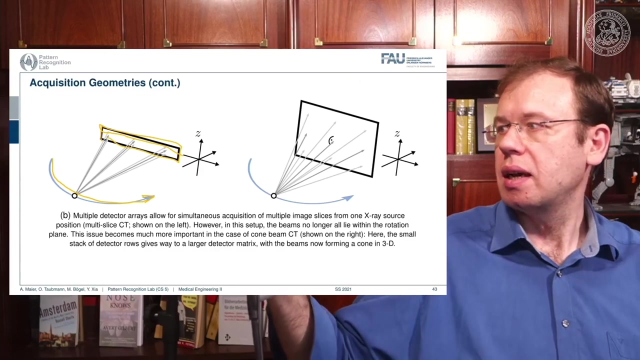 58, 59, 60, 61, 62, 63, 64, 65, 67, 68, 69, 70, 71, 72, 73, 74, 75, 76, 77, 78, 79, 80, 81, 82, 83, 84. 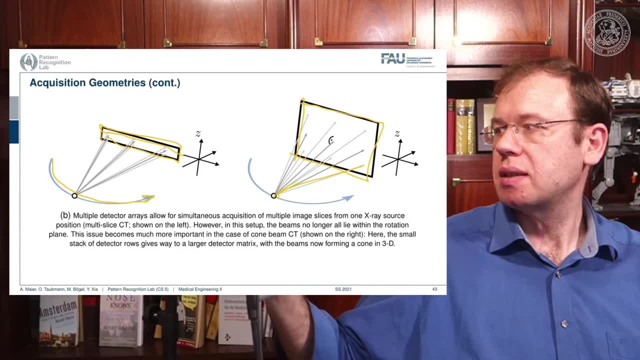 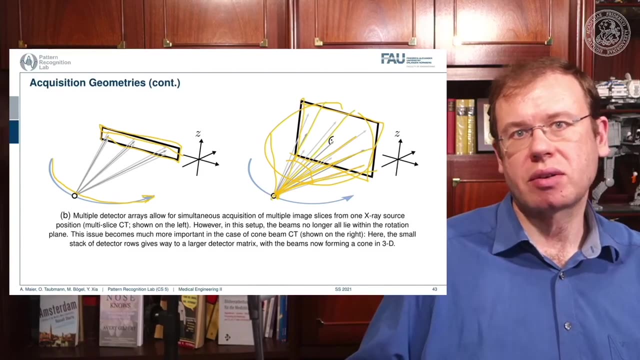 85, 86, 87, 88, 89, 90, 91, 92, 93, 93, 94, 95, 96, 97, 97, 98, 100, 10, 10, 11, 12, 13, 14, 15, 16, 17. 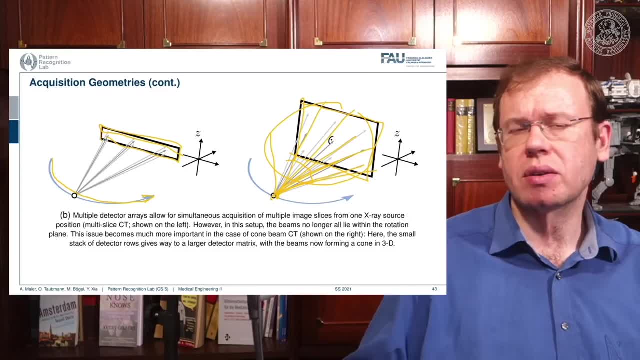 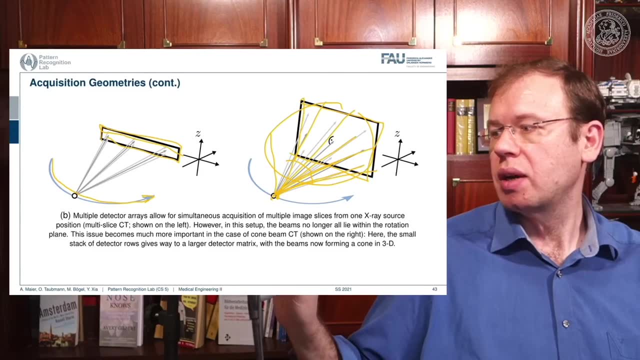 18, 19, 20, 21, 22, 23, 24, 25, 26, 27, 28, 29, 30, 31, 32, 33, 33, 34, 35, 36, 37, 38, 38, 39, 40, 41. 42, 43, 44, 45, 46, 47, 48, 49, 50, 51, 52, 53, 53, 54, 55, 56, 57, 68, 69, 70, 71, 72, 73, 74, 74, 75. 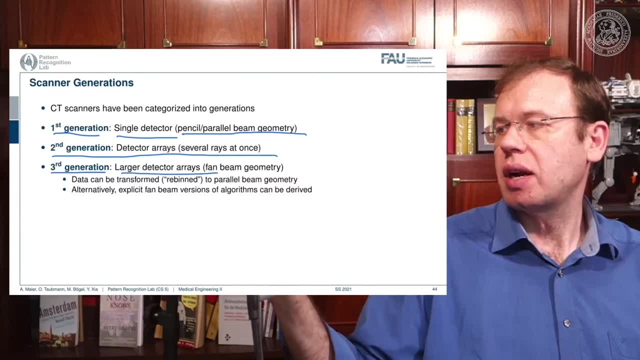 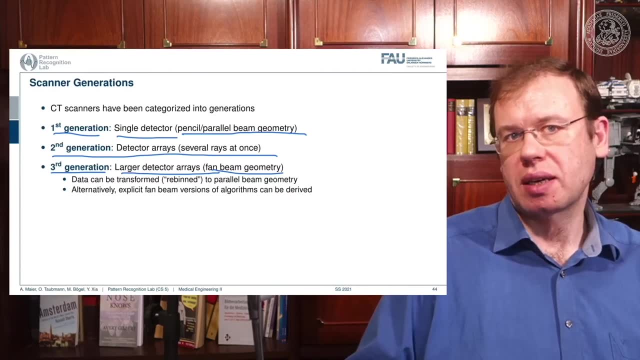 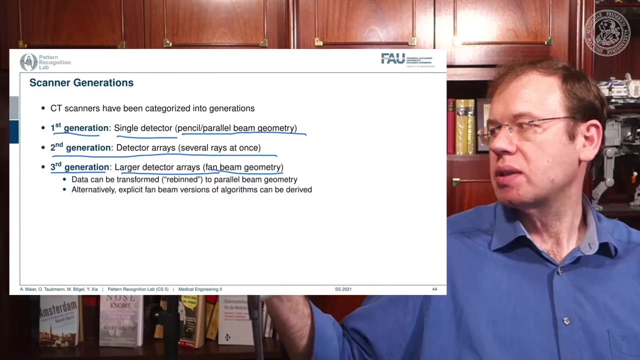 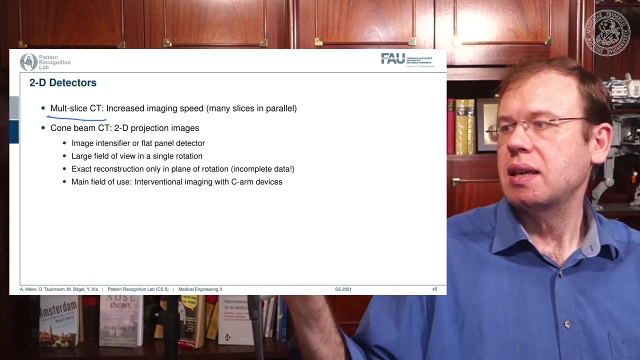 75, 76, 76, 77, 78, 78, 79, 80, 81, 82, 83, 84, 85, 86, 87, 88, 89, 90, 91, 92, 93, 93, 94, 94, 95, 96. 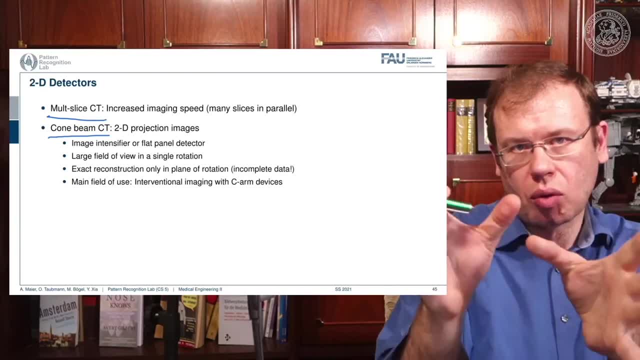 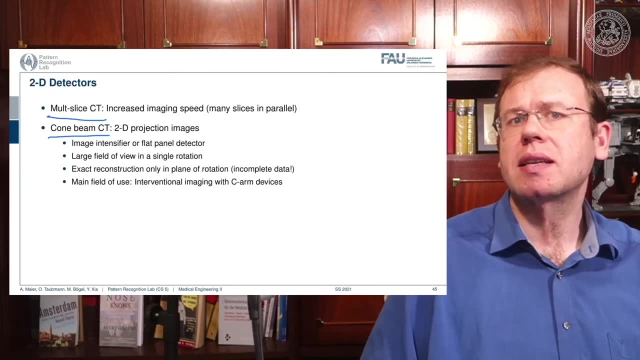 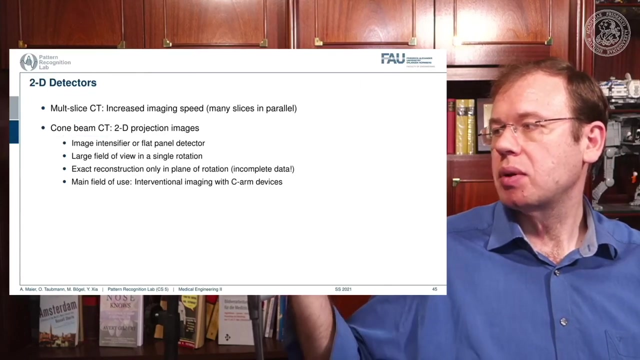 97, 97, 97, 97, 97, 98, 100, 12, 13, 14, 15, 16, 17, 18, 19, 20, 22, 23, 24, 25, 26, 27, 28, 29, 30, 31. 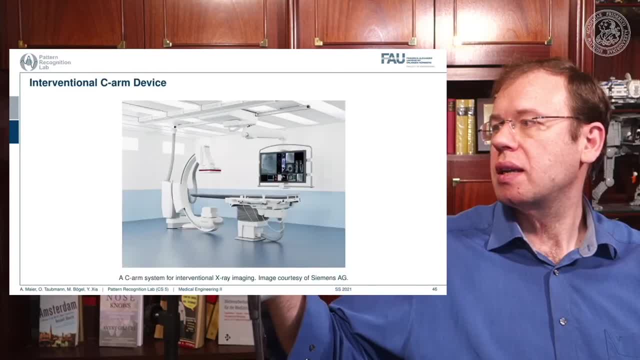 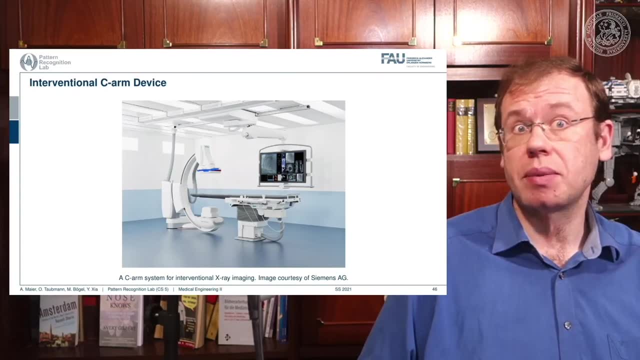 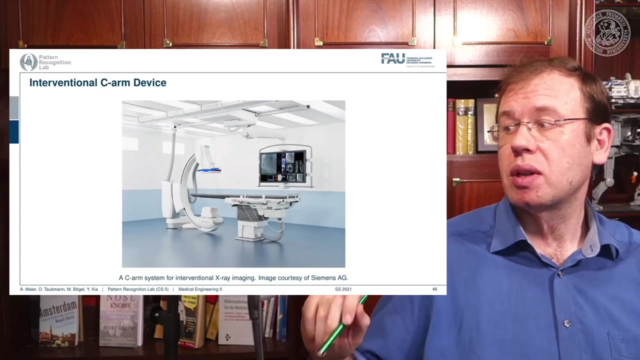 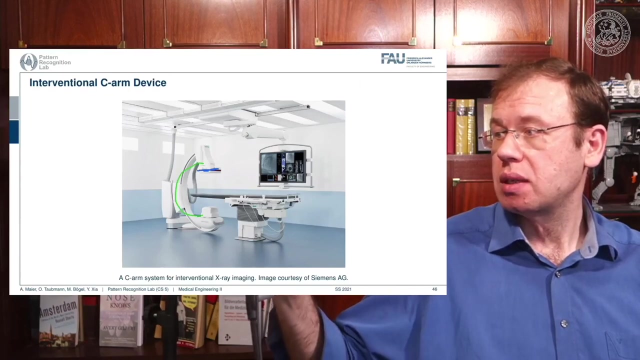 23, 24, 25, 26, 27, 28, 29, 30, 31, 32, 32 And because we now have the mathematics to solve also combium acquisitions, we can also compute 3D images in the operation room. So you essentially take the system and rotate it about this axis here. 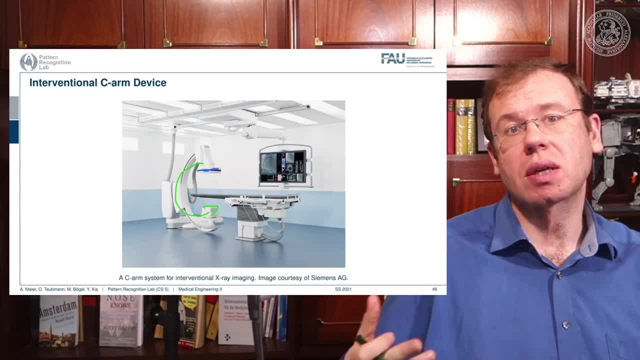 and then you have a CT acquisition and you can reconstruct entire volumes directly at the place of surgery, And that's really cool for a neurosurgery. then you can really get 3D reconstructions of the vessel tree of the patient on the table. 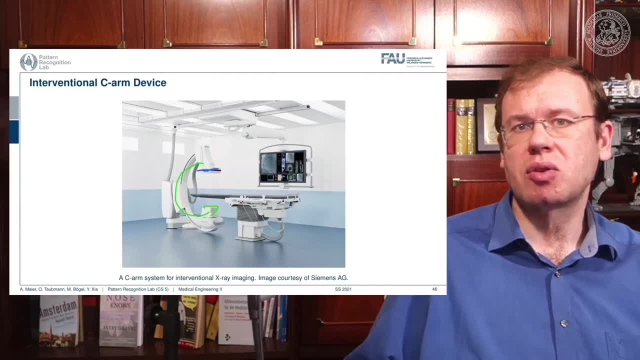 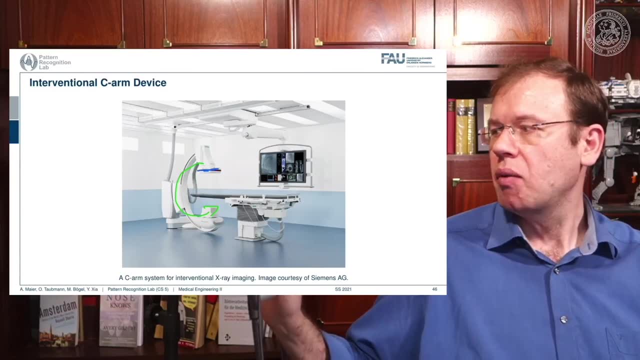 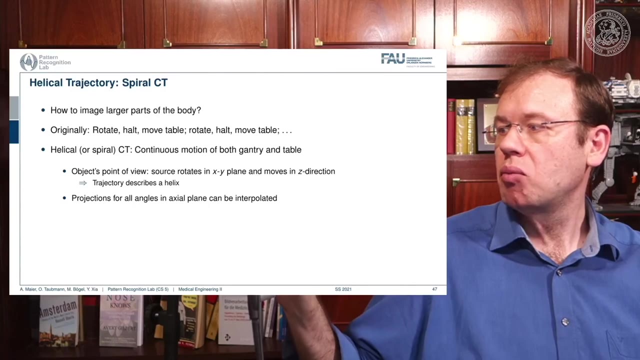 in close to real time, So it takes about 20 to 5 seconds to perform such a scan, and then you have a complete 3D memory. So this is pretty cool. Well then, the famous helical CT is that you now start moving the patient. 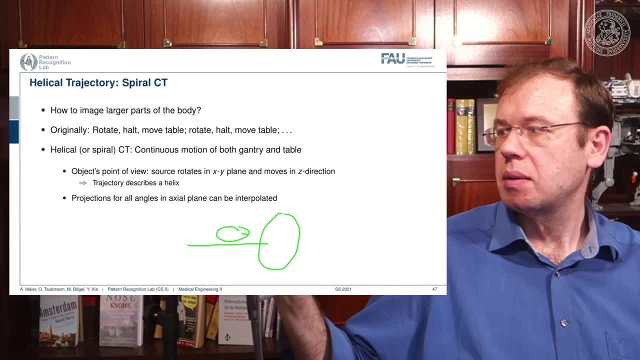 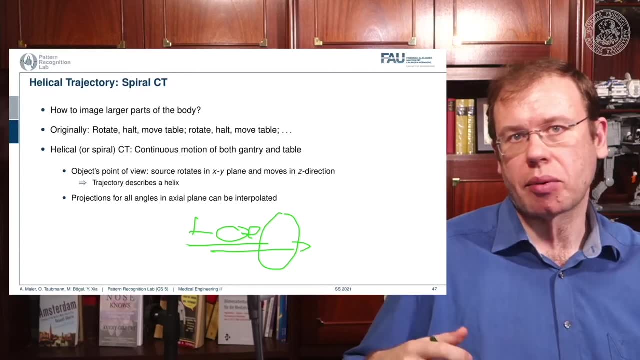 So if this is the gantry, you have the patient and the patient is lying here. So you start moving the patient through the gantry at an appropriately set time. So you start moving the patient through the gantry at an appropriately set speed. 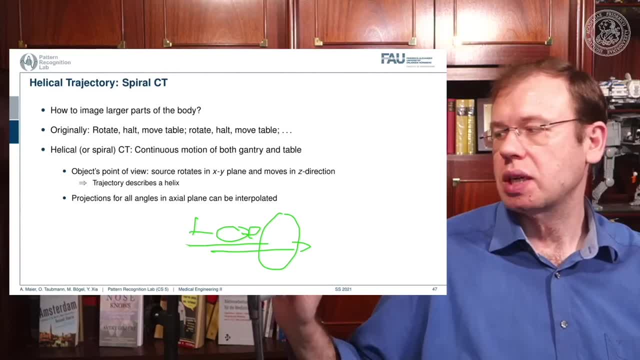 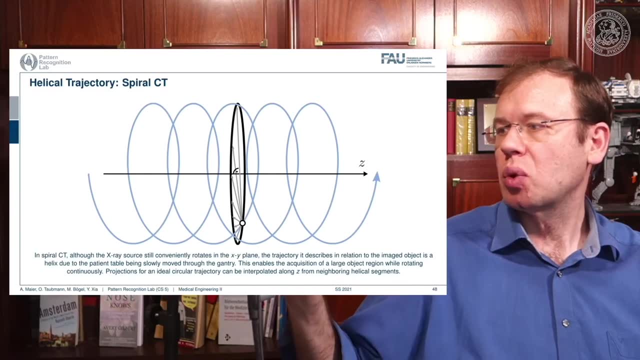 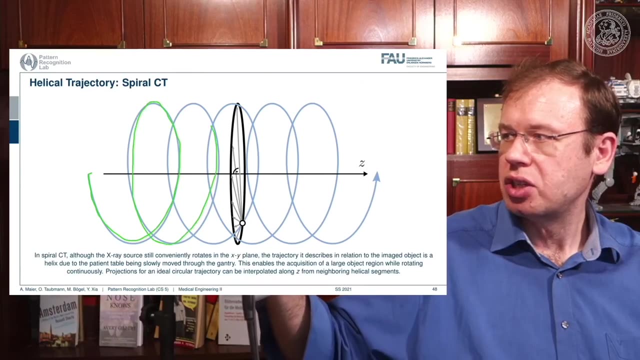 And this allows us to reconstruct all of the points of the patient at once And it is a complete trajectory. So this gives them rise to trajectories that look like this, So you can think of the actual source position with respect to the patient is actually moving on this helix here, because we're moving the patient with respect to the source. 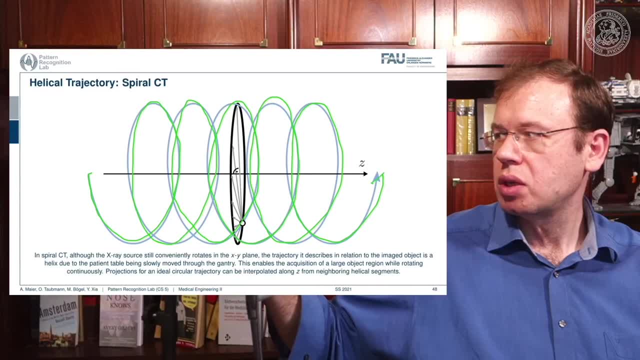 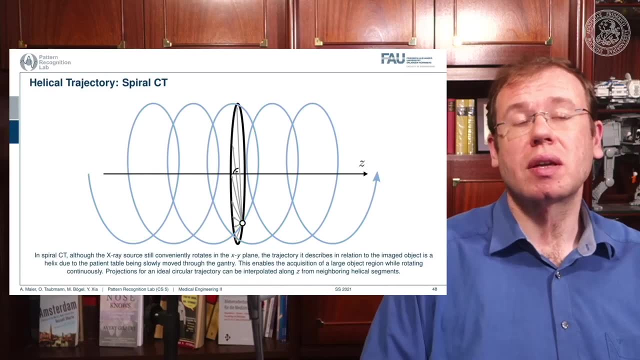 And this gives us this kind of helical- or you could also say spiral- motion, in order to acquire everything At once and this is really complete and you can reconstruct, without larger artifacts or missing data, the entire 3D volume of a whole body scan. 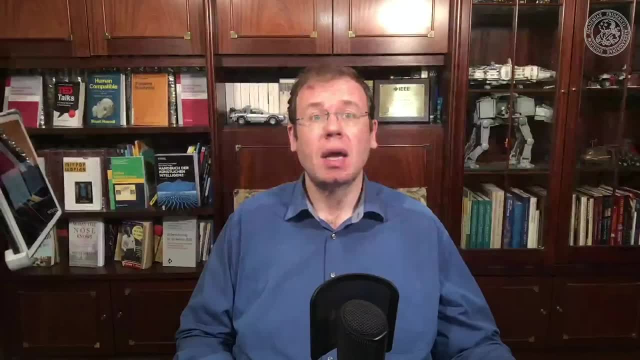 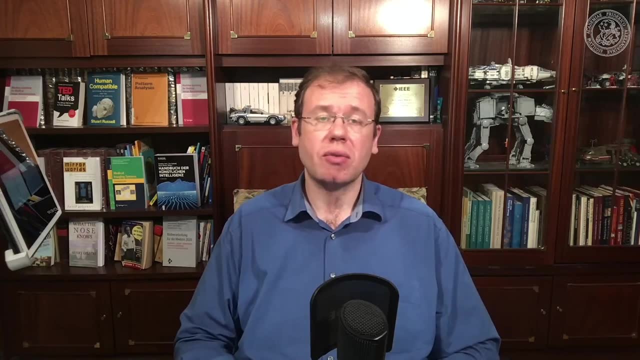 So that's really a really cool technology. Well, this already brings us to the end of this video, So you've seen here now the two main approaches for imagery construction, That is, the filter back projection rather than inverse type- and also the algebraic approaches.